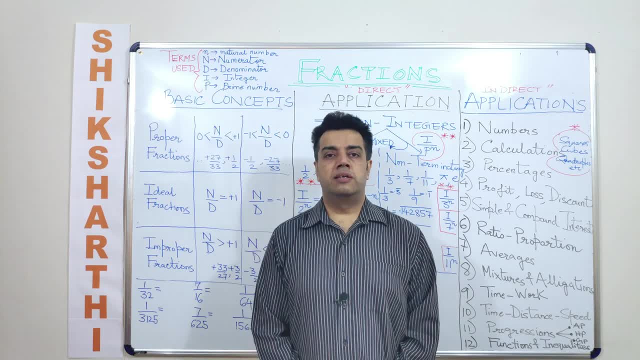 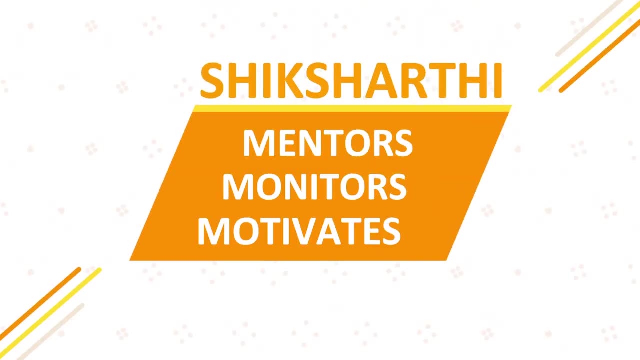 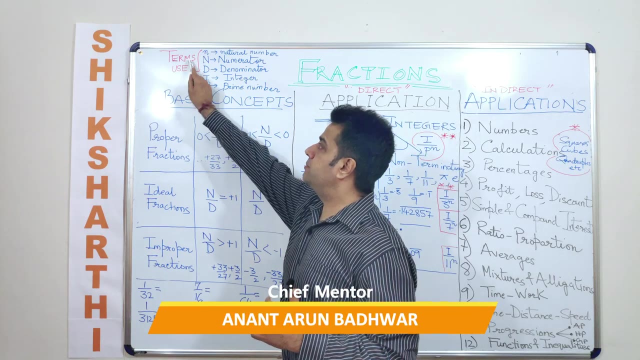 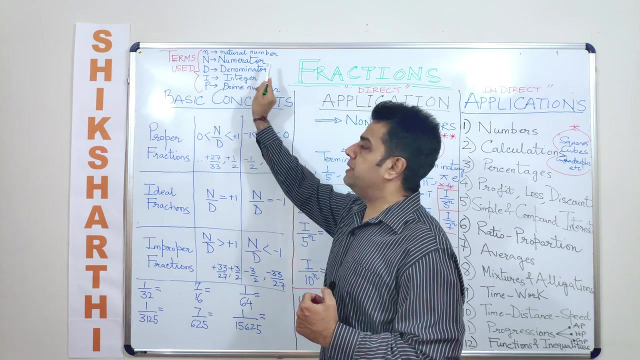 Hello friends, welcome to Shiksharati. In this session, we will be talking about fractions. Okay, before we go ahead, these are some terms that I have used on this whiteboard, the full form of which has been written here Now. small n means I am talking about a natural number. 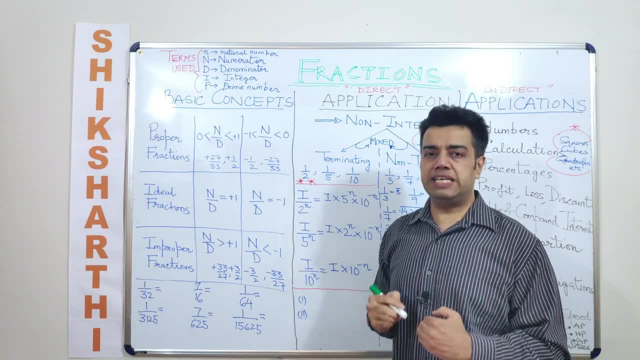 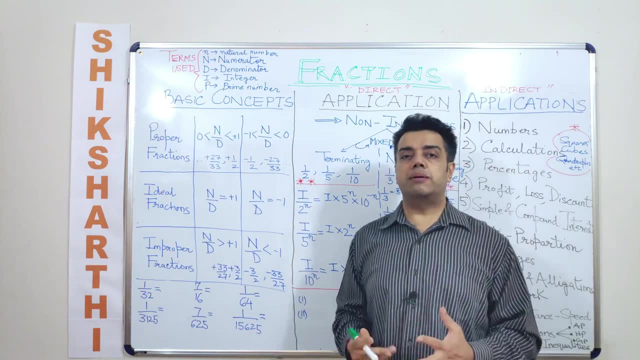 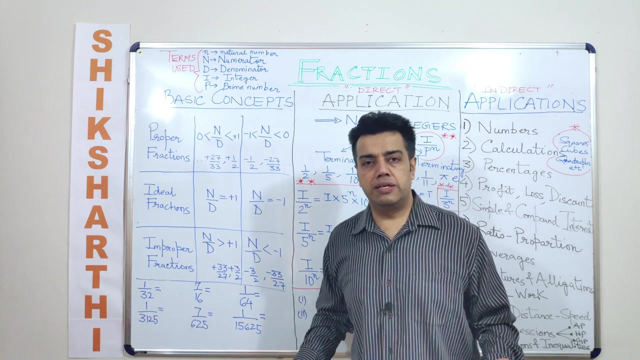 capital. N means I am talking about the numerator capital, D is denominator capital. I is an integer. I hope you know what is an integer. An integer is a number which is written without a decimal point. For example, 100,, 200,, 300,, 1,, 2,, 3,. all of these are integers. only Why? Because 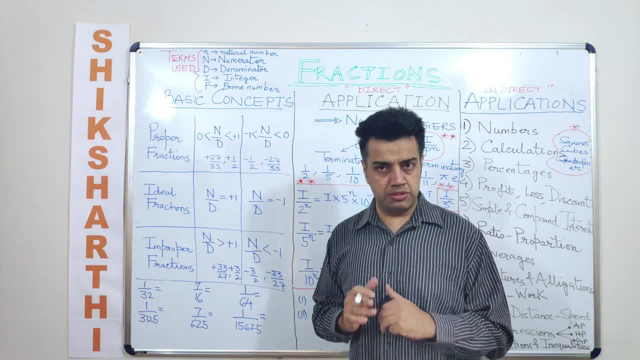 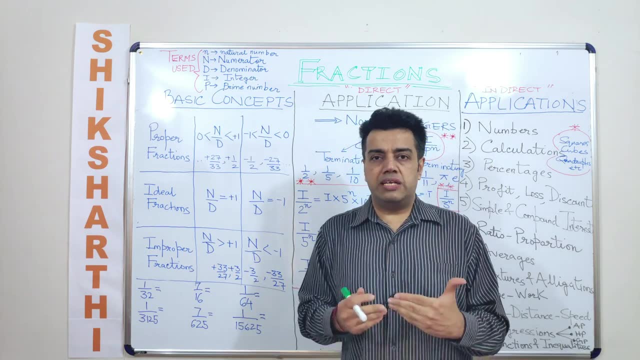 they are written without a decimal point, right? And then P is for prime numbers. What are prime numbers? Prime numbers are the numbers which are written without a decimal point. So prime numbers are those numbers which are divisible by exactly two factors, and those two factors are 1 and the. 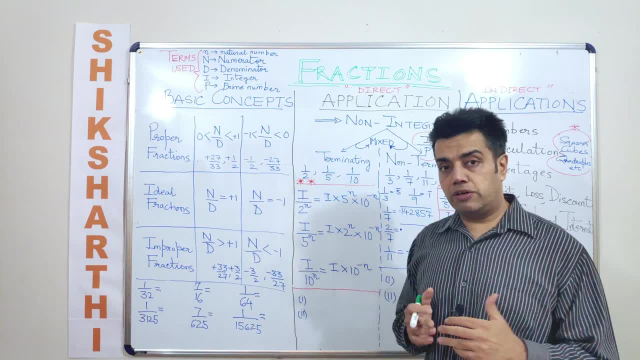 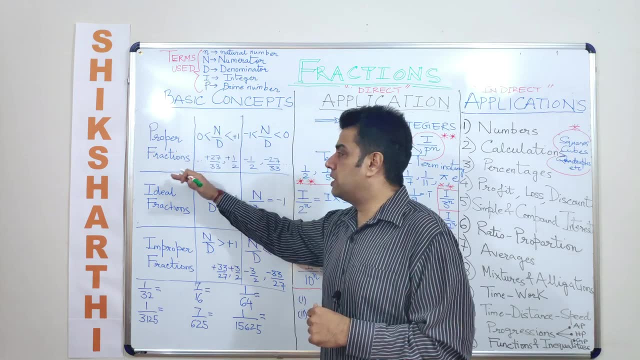 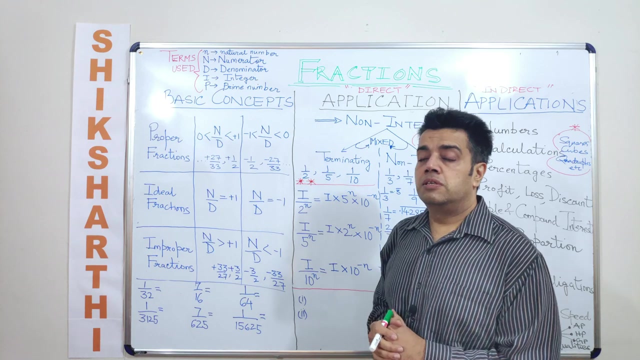 prime number itself. Okay so, starting off with the agenda for the day, which is fractions. Okay so now the fractions are broadly divided into three parts. broadly So, what are different types of fractions? Proper fractions, ideal fractions and improper fractions. 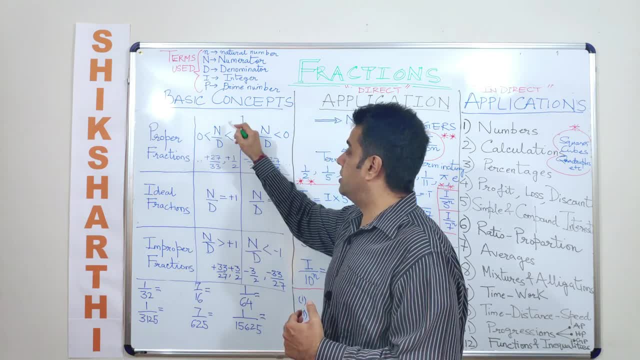 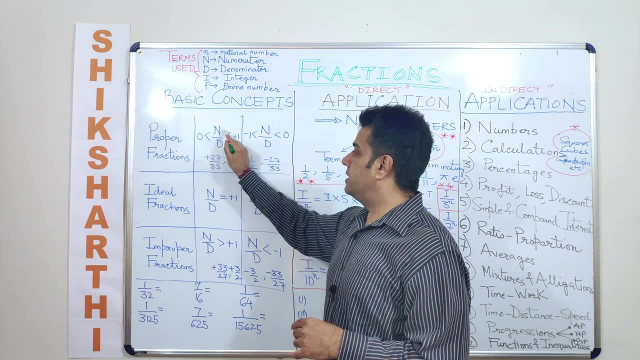 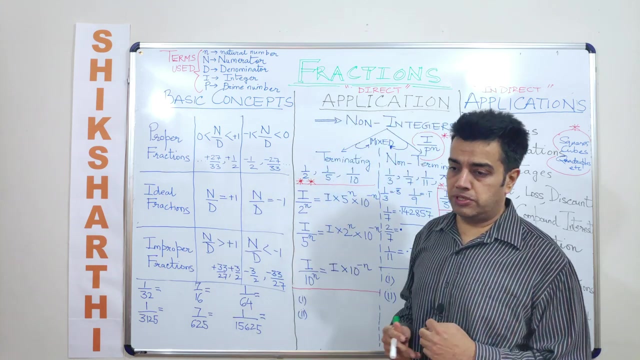 Now proper fraction is: I have taken a fraction in the format of a fraction, which is a numerator divided by a denominator. So when I say a numerator divided by a denominator lies between a 0 and a 1.. Again, let us lay emphasis on the words being used. I am talking about between. 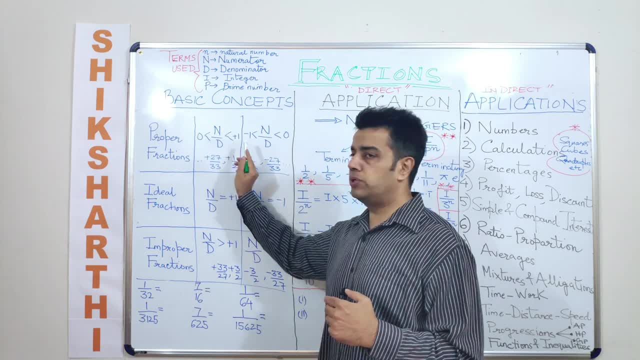 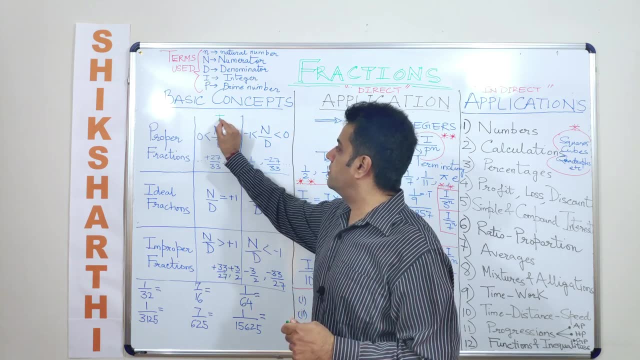 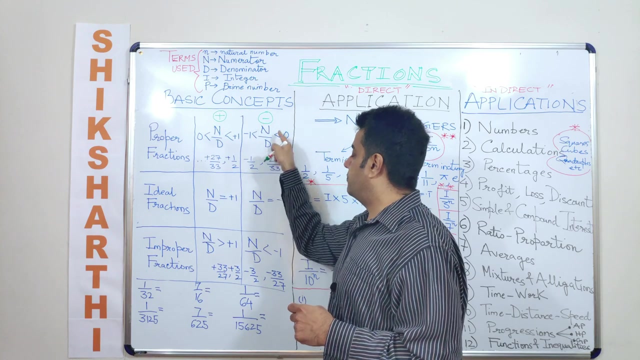 Between means that the extreme values are excluded. They are not included. Similarly, this is a positive, proper fraction. So this we are talking about positive side of it and this we are talking about the negative values. So if I say, if there is a, 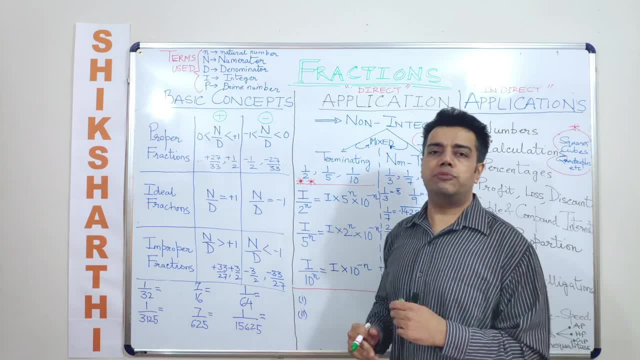 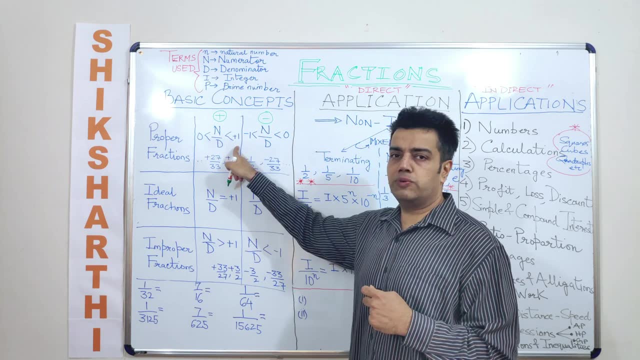 fraction which lies between minus 1 and 0, I am talking about a negative proper fraction, The examples of which are written here Now: 27 divided by 33 lies between a 0 and a 1.. So it will be. 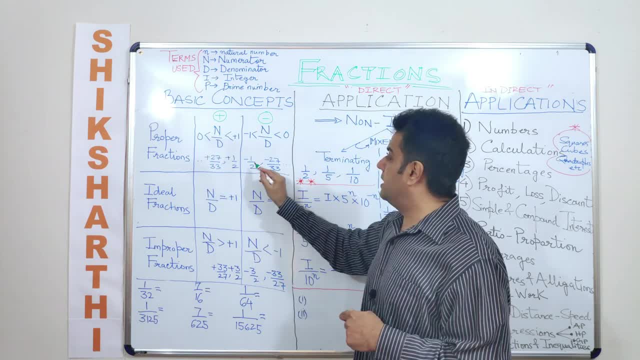 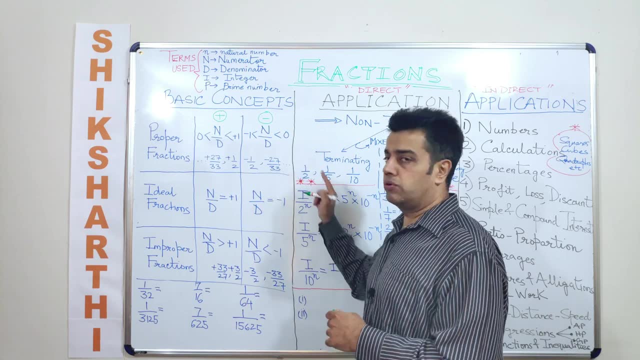 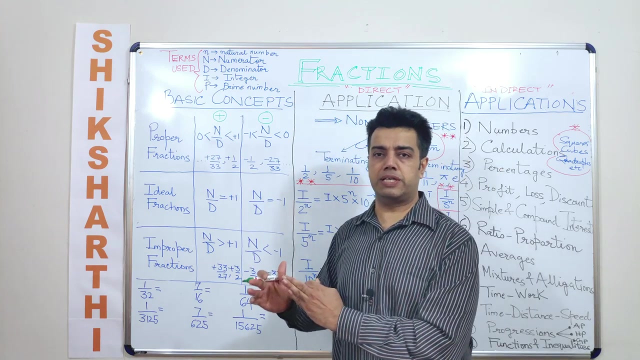 termed as a proper fraction, Same for 1 by 2.. Similarly, if I take a fraction like minus 1 by 2 or minus 27 by 33, these are two different values and many more. Such values which lie between minus 1 and a 0 will be known as negative proper fractions. 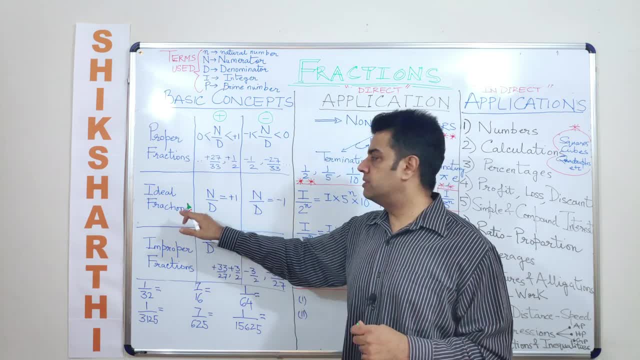 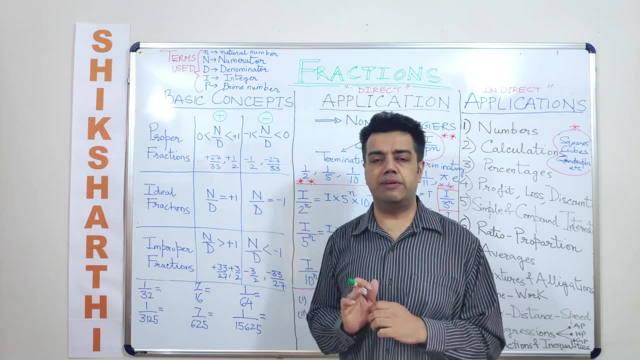 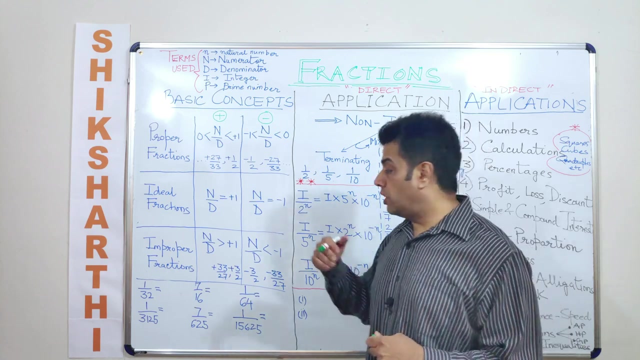 Next is ideal. So when I am talking about ideal fractions, I am basically talking about: plus 1 is a positive ideal fraction and minus 1 is a negative ideal fraction. There is or there are no other values other than these, Right? So now, when I talk about improper fractions, 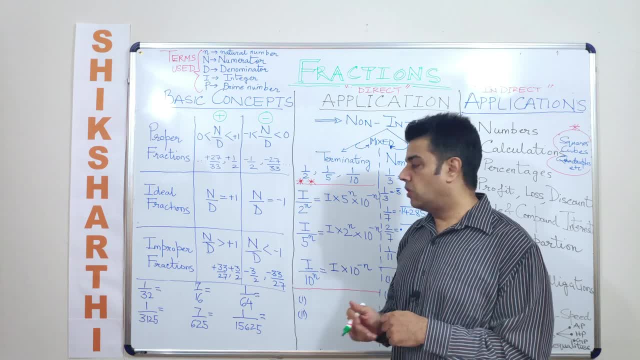 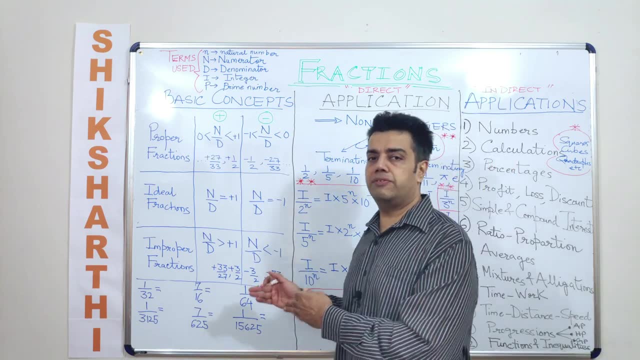 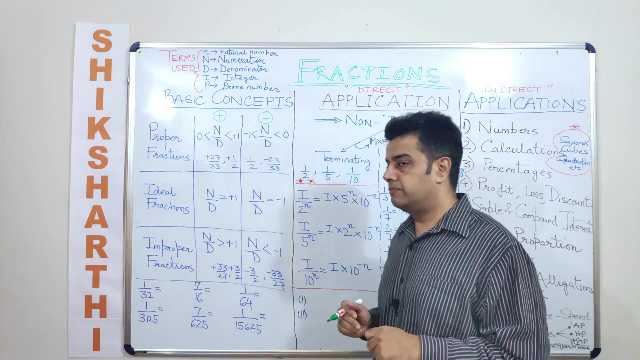 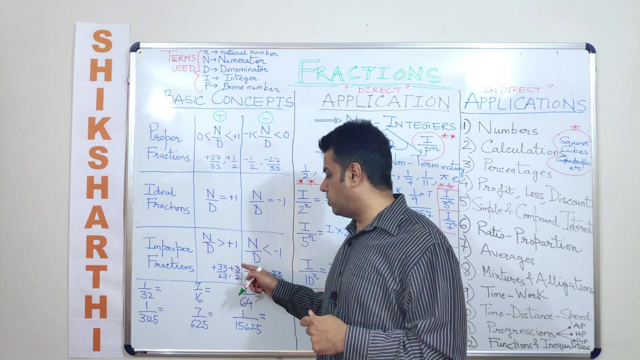 any fraction which is greater than plus 1, or any fraction which is less than minus 1 will be termed as either positive improper fractions or negative improper fractions. Let us lay emphasis on the word either, which I have discussed in some other video as well. Okay, So if I take a fraction like 33 by 27 or 3 by 2 will be termed. 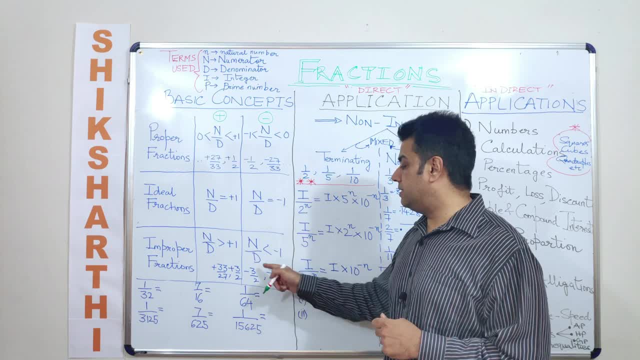 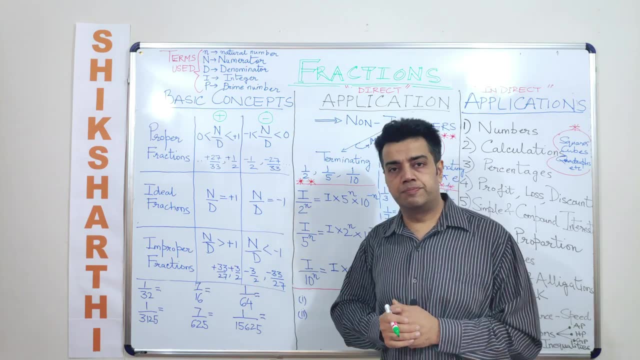 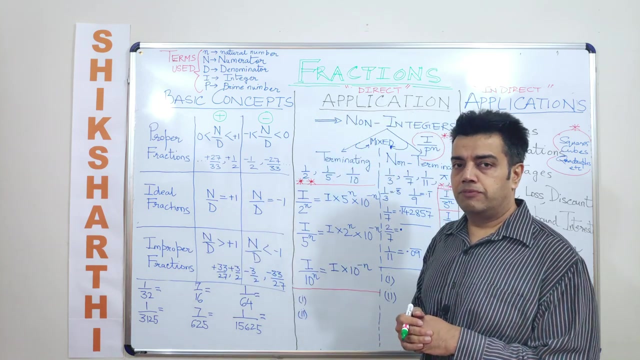 as a positive improper fraction by definition. Similarly, minus 3 by 2 and minus 33 by 27, will be termed as a negative improper fraction by definition. Right Now, once these basics are clear, then we can take it to a next level. For example, there are many more terminologies. 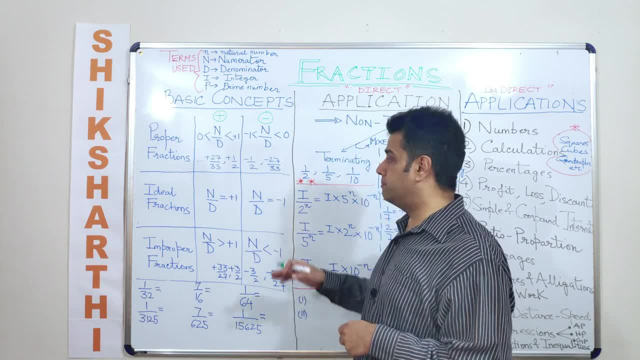 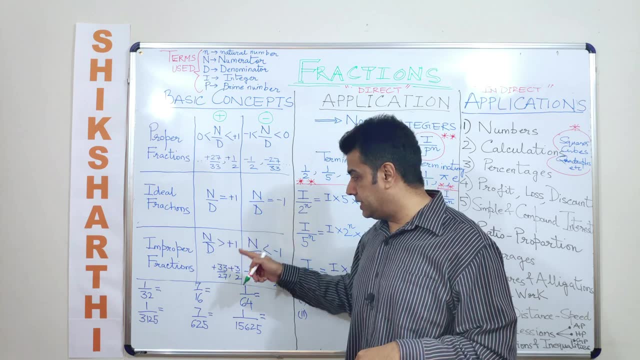 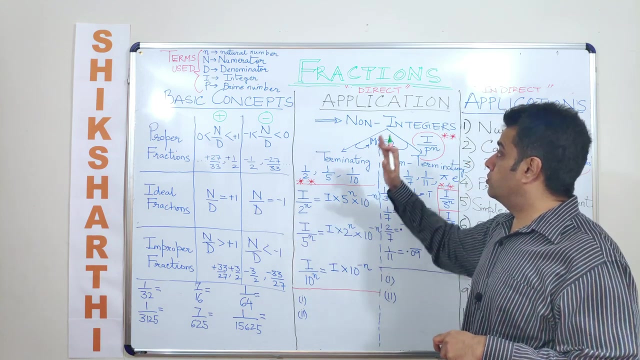 which are used for fractions, But I, as I said earlier, also the basic. if I talk about the basic division of fractions, these are the three divisions that I can talk about. Right, Let us come to the next stage, So the direct application of these. the direct applications. 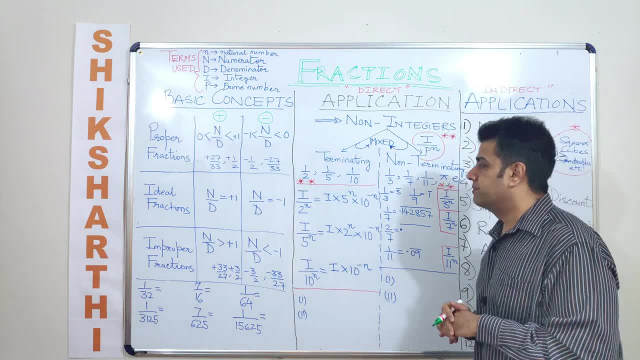 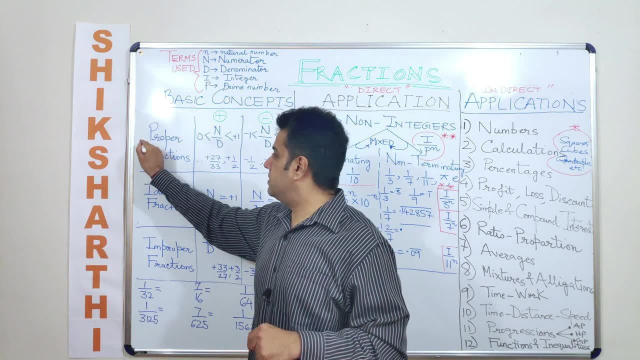 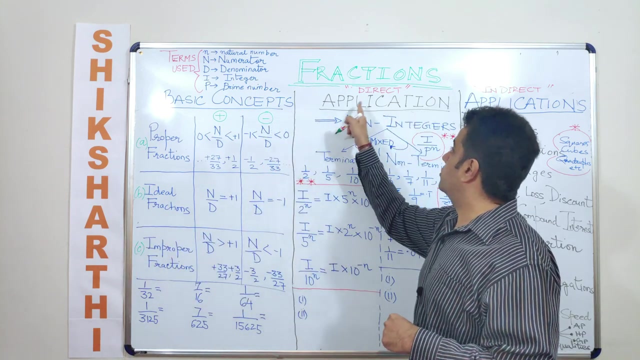 of these three will translate into what. So I would say, now we are basically talking about the application of this and this. So if I label this as A, this as B and this as C, So now we are talking about a direct application of A and C. 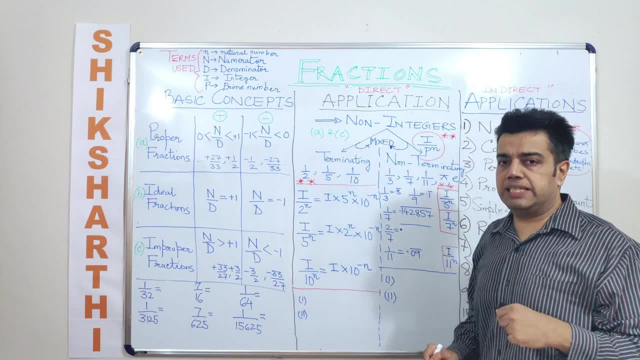 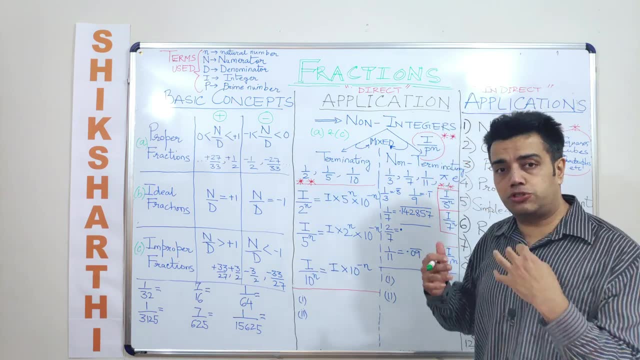 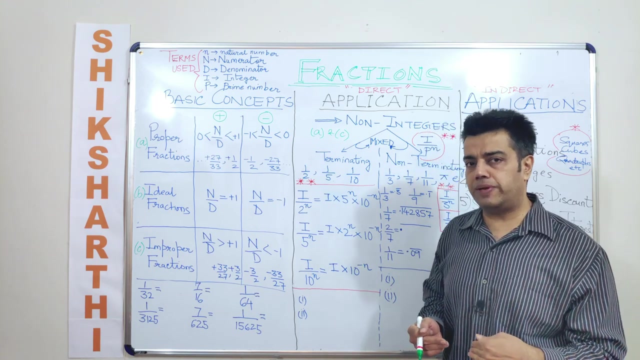 And the direct application is what Non integers. So the first and the foremost application of this chapter or this topic is numbers. So I can get numbers, I can discuss numbers and then I can come down to fractions. Or if I am discussing fractions, it is mandatory. 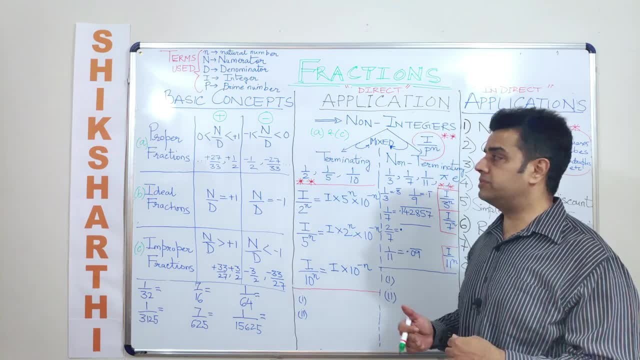 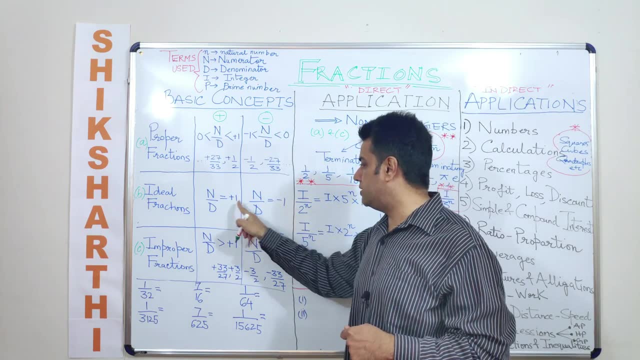 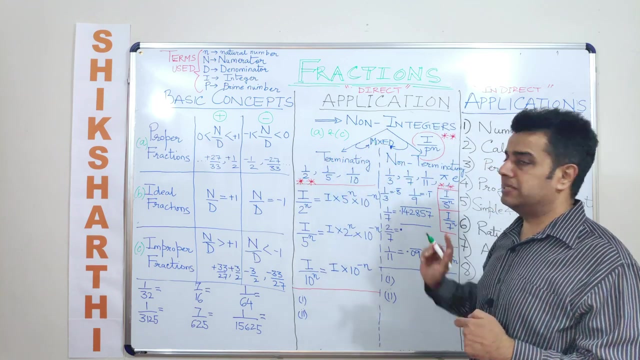 for me to discuss numbers. When I am discussing numbers here now, we started off with integers also, And now we are talking about non integers. So if I talk about these two values, these are integers. Now the remaining two terms: if I talk about term A and term C, we are basically focusing. 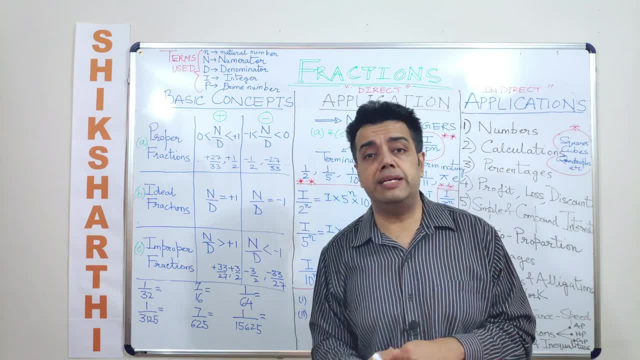 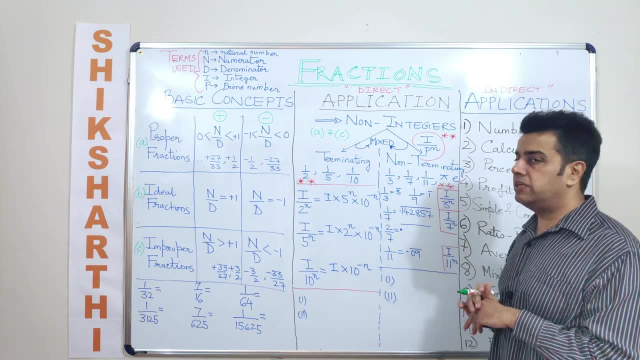 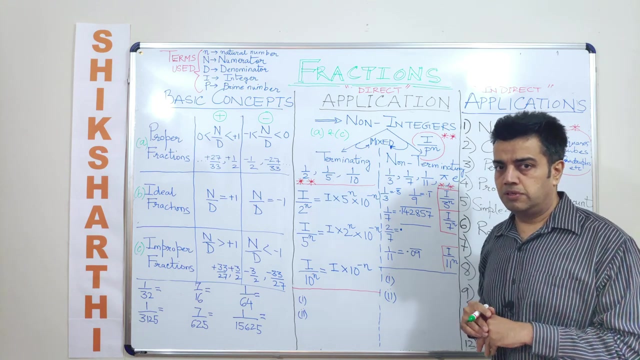 on non integers. Now non integers can be further classified into terminating fractions or terminating non integers, or I can call them as non terminating fractions or non terminating non integers- Confused, Let me revisit. So here I am, dividing the non integers into two different parts. 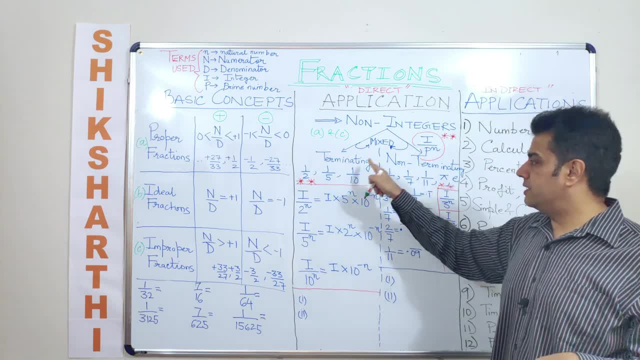 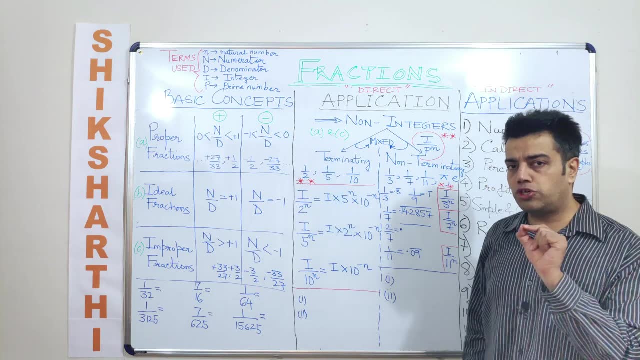 One is the terminating part and the other one is the non terminating part. Terminating means this will give me a value, like, let's say: one by two gives me how much Point five it stops. One by five gives me how much Point two it stops. 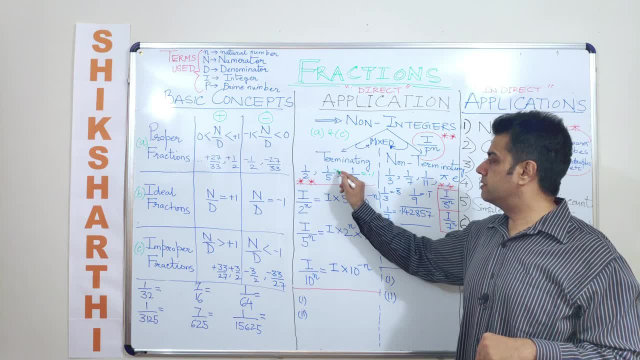 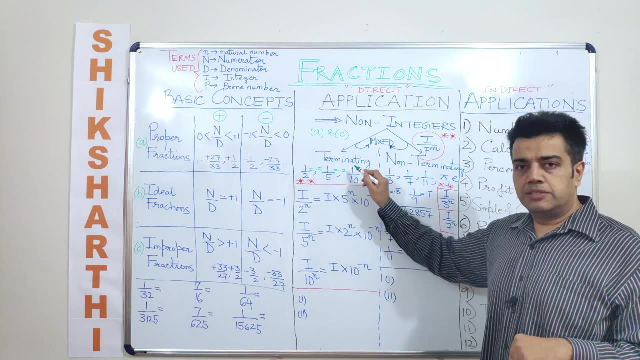 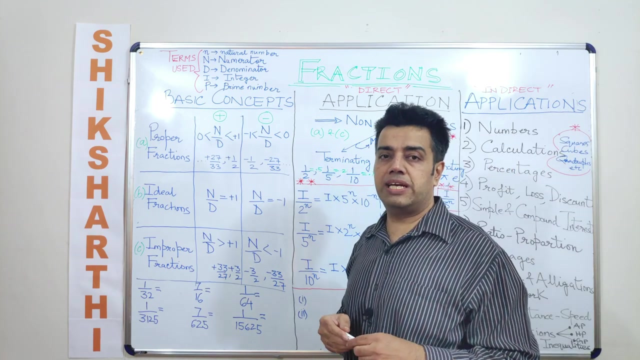 One by ten gives me how much Point one it stops. Now these are terminators, Terminating fractions resulting into a terminating non integer. Now, here, non integer has to be understood as a number with a decimal point. Point is a non integer. 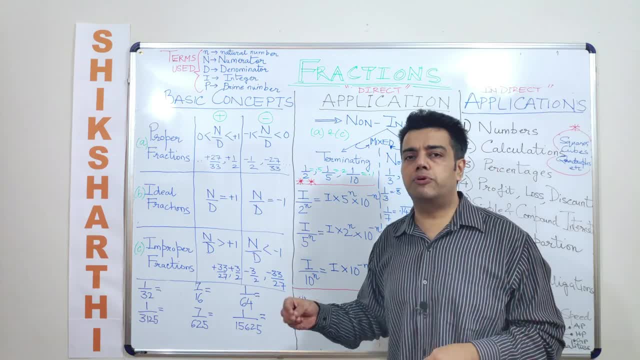 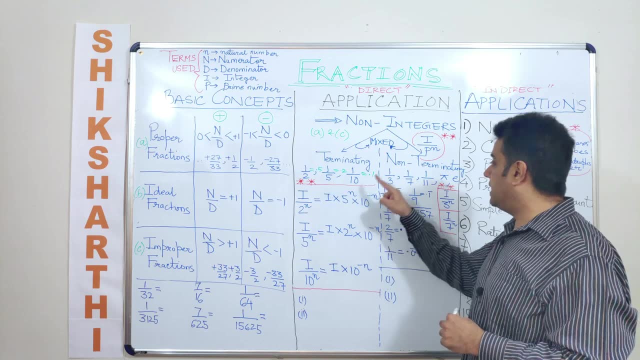 For example, if I'm writing 1.5,, 100.5, 200.5, all of these are non integers- having a terminating decimal. Similarly, I can have a non terminating decimal also. Now, non terminating decimal Terminating. 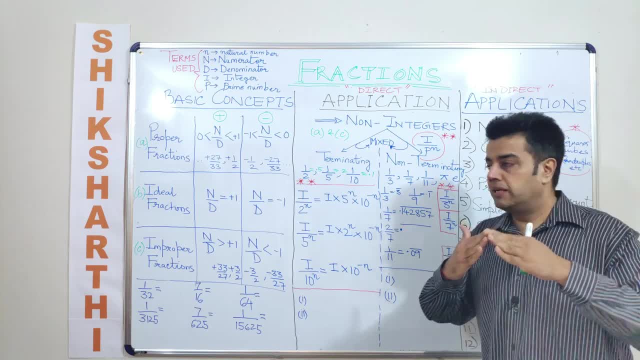 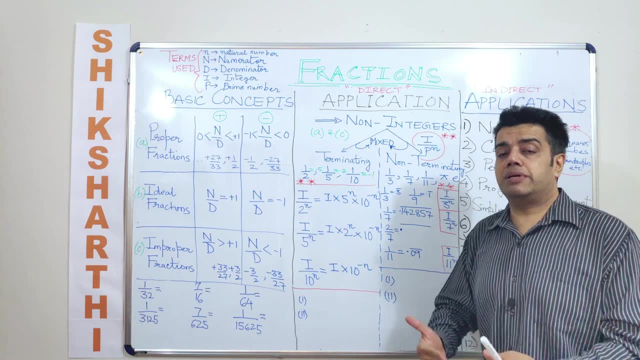 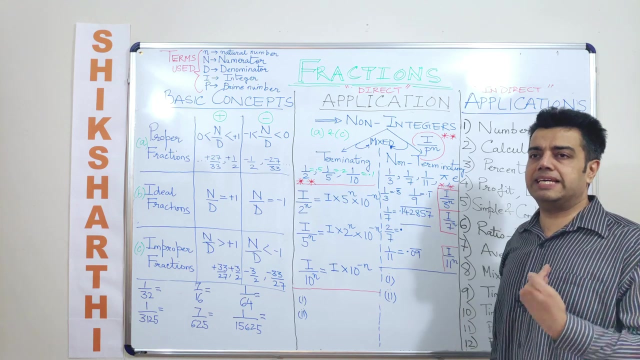 Decimals again can be divided into two parts. One part is I talk about these three wherein I am getting a recurring decimal. Now, when I say one by three gives me a point three: recurring. This bar shows what it is: a recurring decimal, which means it can also be written as point. 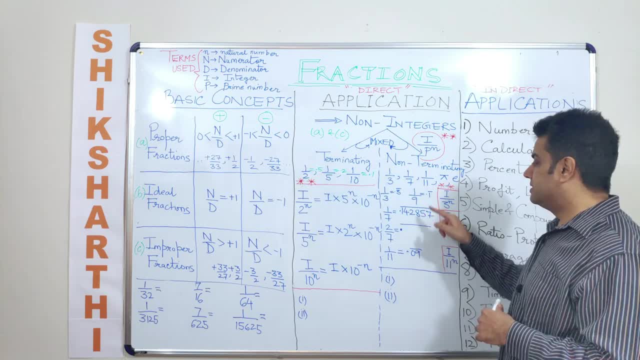 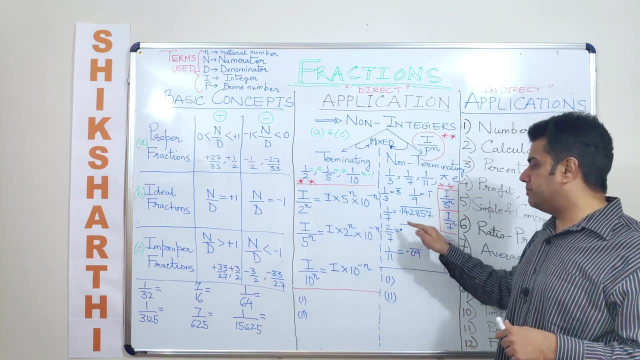 three, three, three, three, three, three, and so on. Similarly, one by nine can be written as point one: one, one, one and so on. Similarly, one by seven can be written as point one: four, two, eight, five, seven, one. 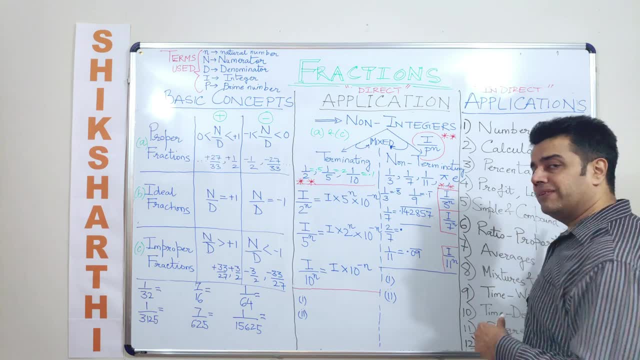 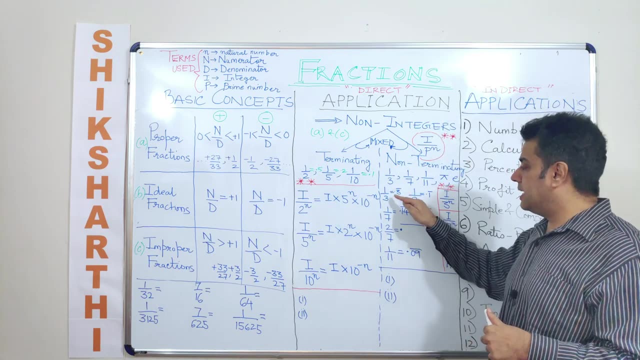 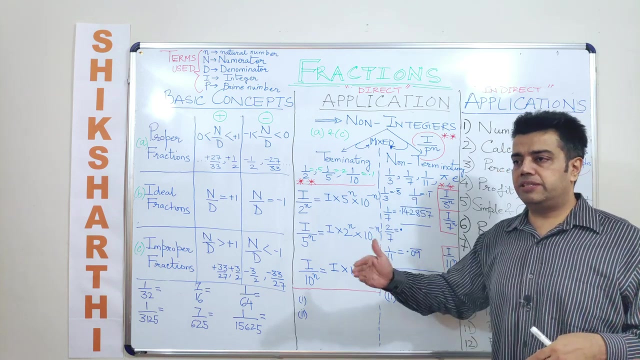 four, two, eight, five, seven, one four, two, eight, five, seven, and so on. right, So now here you will see that the non integer part has a definite time period of repetition. I mean, if I'm writing this as point three, three, three, three, three, it will repeat: 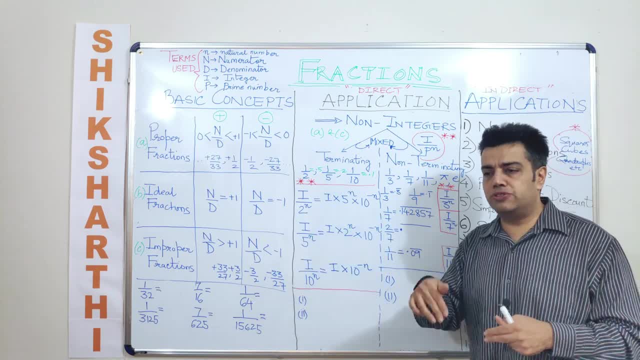 after one, one value. Or let us say there is no difference in time. Let us say there is no difference in time. Let us say there is no difference in time, Let us say there is no difference in between. So there is a definite time period of repetition. 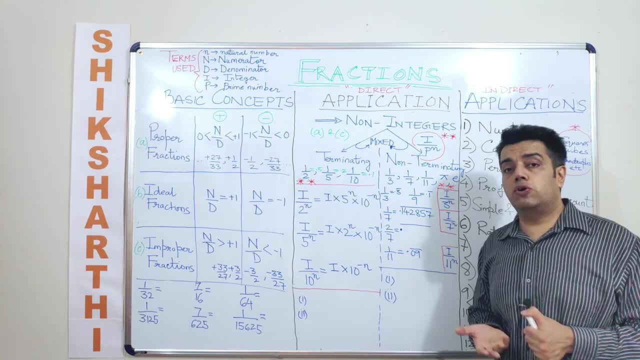 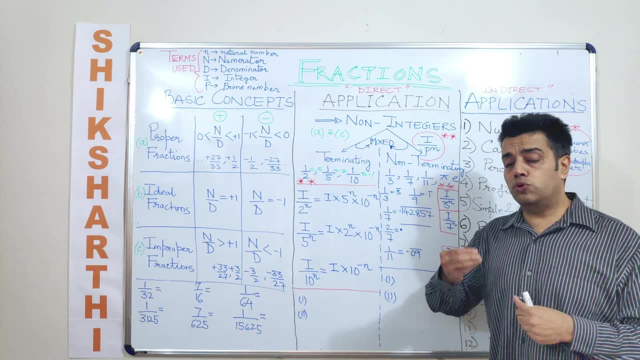 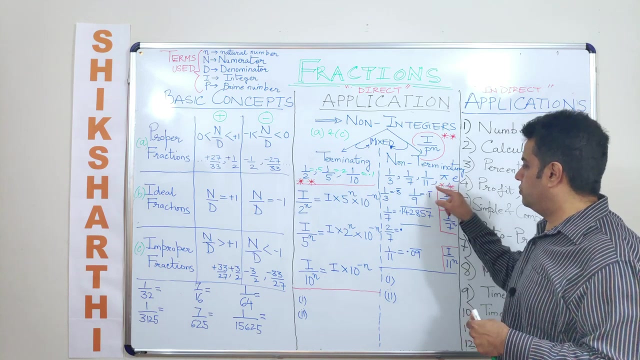 Then there are terms as pi and e, which are also known as I mean they have a non terminating decimal, but then they do not. those decimal points do not come with a fixed time period of repetition. For example, you know, pi can be written as three point, one, four, two, followed by maybe. 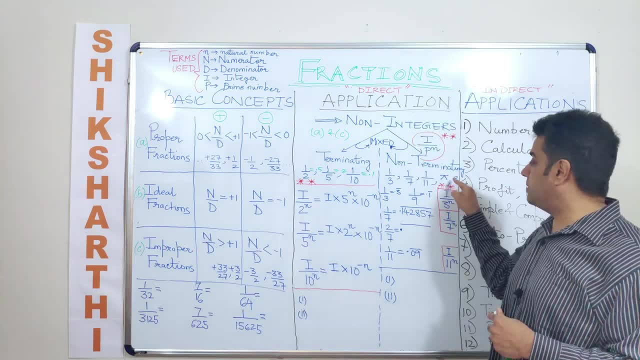 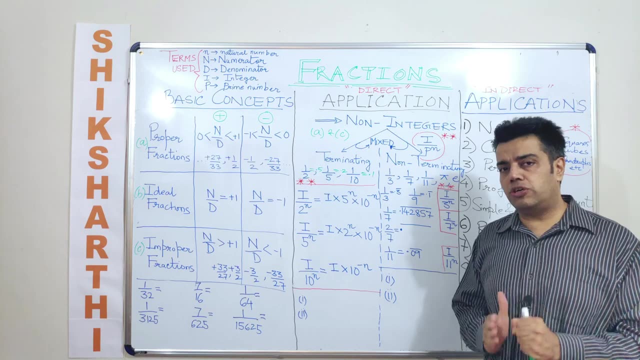 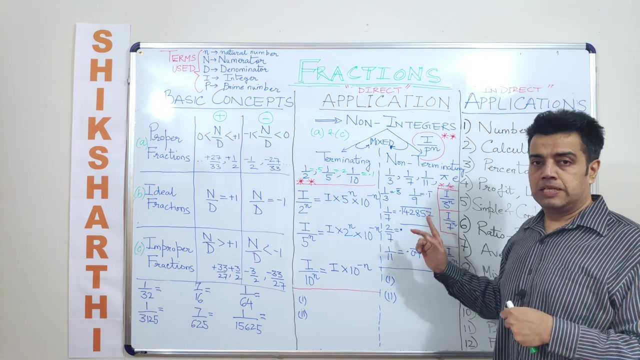 a one four followed by a three. So this will not be a recurring decimal, right, I'll call it as non terminating. but then it is not neither terminating nor it is recurring. So just to cut it short now: non integers can be broadly divided into two parts. 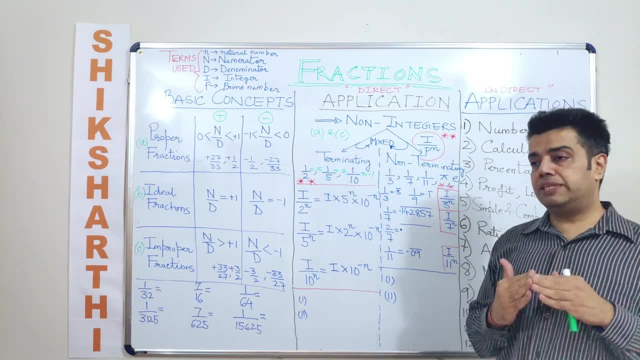 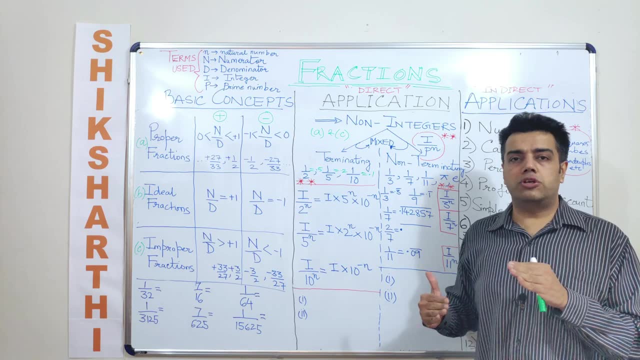 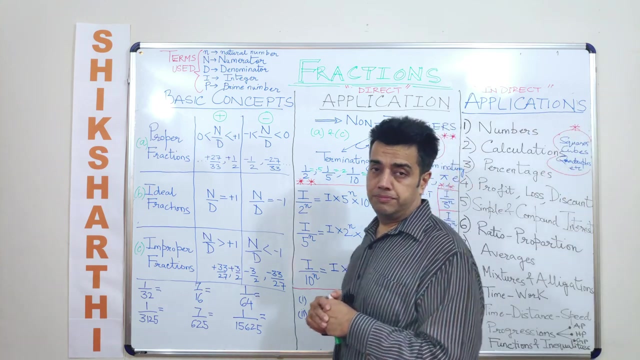 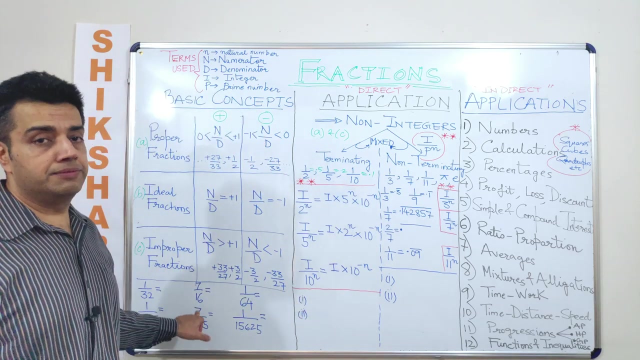 One is terminating and the other one is non terminating. Non terminating can be further understood as recurring- and the second part is some special cases Under non terminating, special cases like pi and e right. Taking it forward Now, when I take it forward, you will see that there are few questions that I have written. 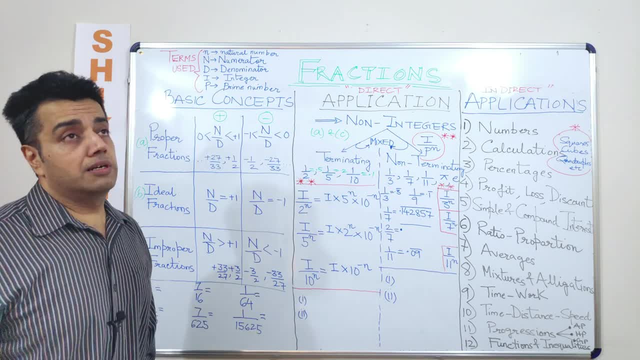 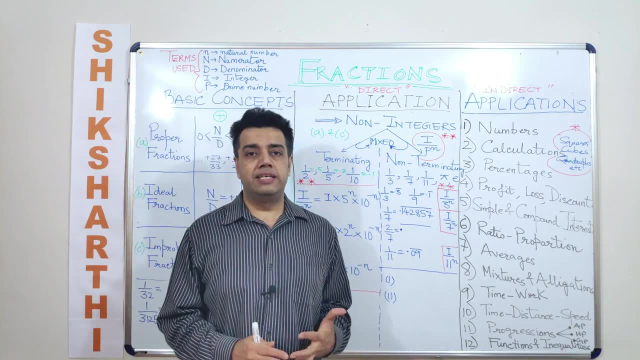 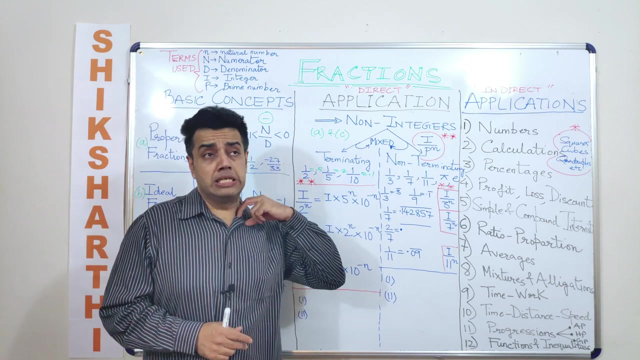 here. These are some questions and generally I see that I mean as a student also. I have come across I being advised to mug up, mug up what? What is the value of one by two? What is the value of one by four, one by eight, one by 16,, one by five? 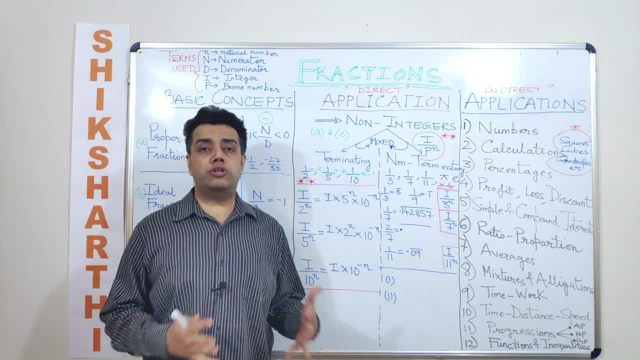 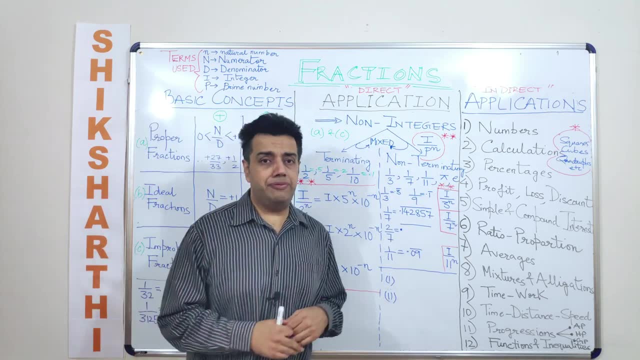 So now my counter to this is: I have always been advising not to mug up. Why? Because this puts me to a discomfort. because if you tell me to mug up all these things even before I write the exam, I feel defeated. What if, if I forget, because I have mugged up? so things go for a toss. 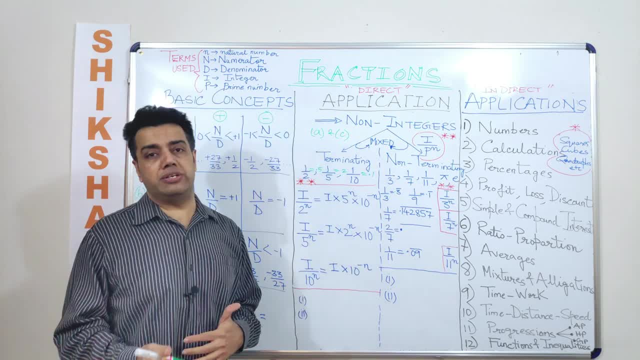 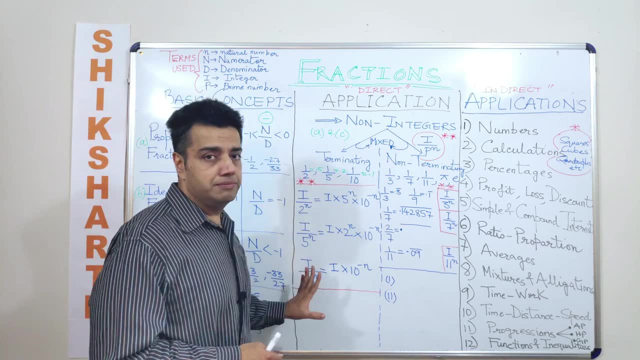 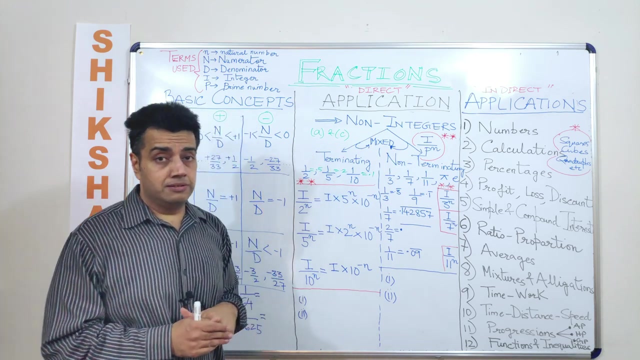 So then there should be a method behind it. So I'm going to discuss the method behind it. So the method says: When will a fraction always give me a terminating decimal? When will a fraction give me a terminating non-integer? So there is a formula for this. 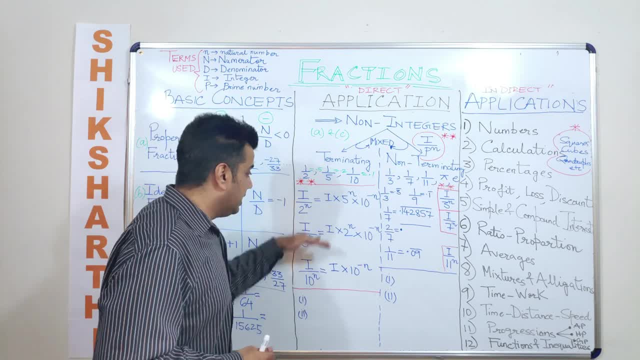 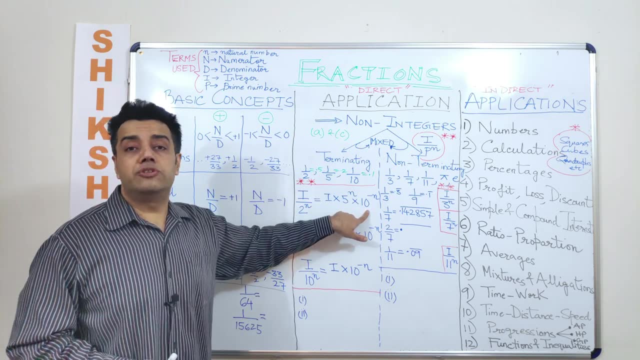 What is the formula? This comes with a lot of efforts here. The formula is: i upon two to the power n can be simply written as: i into five to the power n, into ten to the power minus one. I mean minus n, to be very frank here. 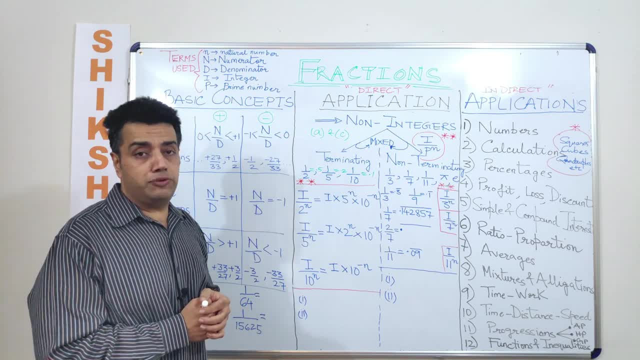 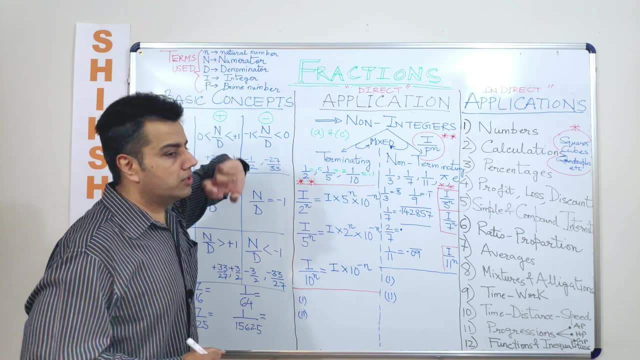 Similar to this. Similarly, i, divided by five to the power n, will be written as i into two to the power n, into ten to the power minus n, where small n is what A natural number. Similarly for this, How to use it. 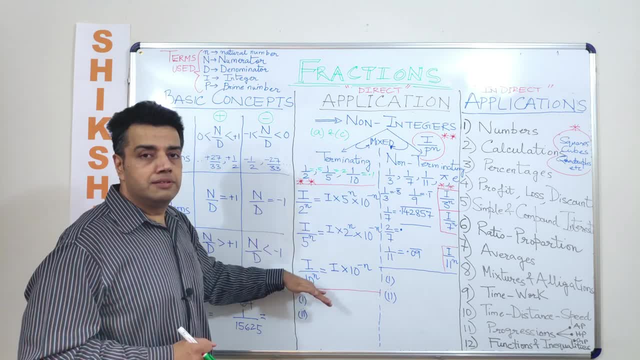 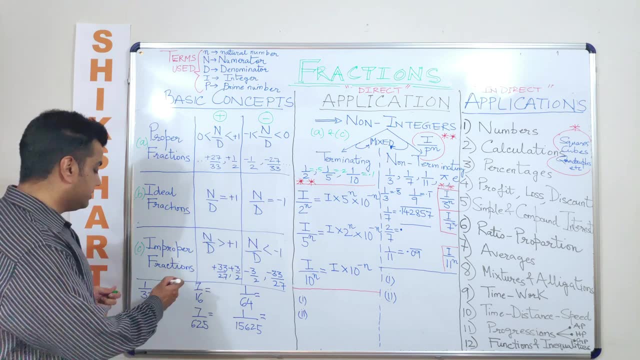 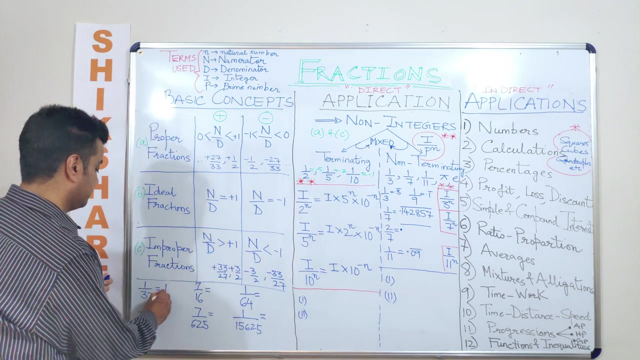 Now, once I know this concept, I can take it to a next level. So if I say one by 32 is nothing but one divided by two to the power five. Now, the moment I'm able to say this, that means this directly translates into what: 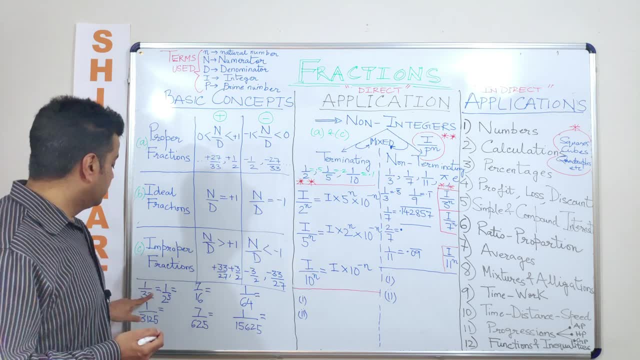 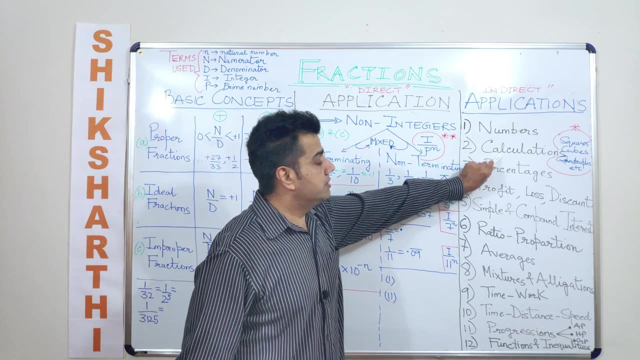 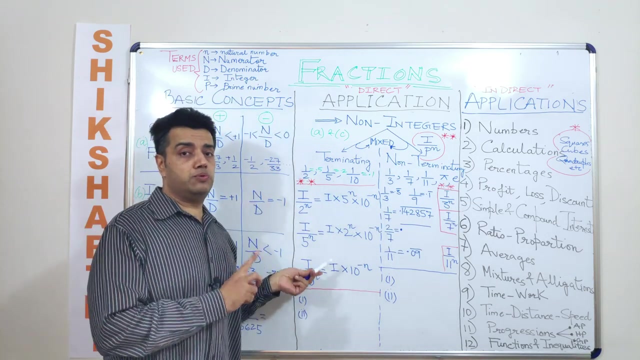 What is the value of? i here one, So I simply need to know or I need to calculate. So, which is why you would see, calculations are important or calculations is an important ingredient. when I'm doing fractions as well, Numbers was always an important ingredient because the direct application was numbers. 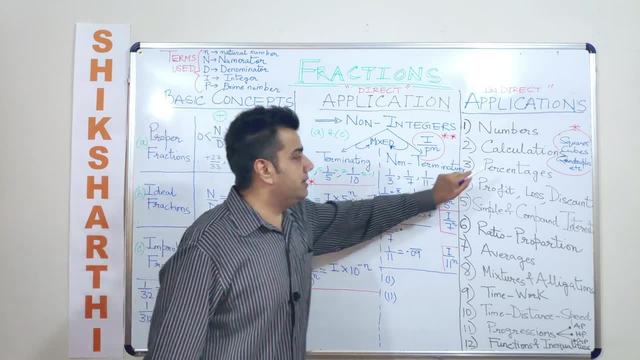 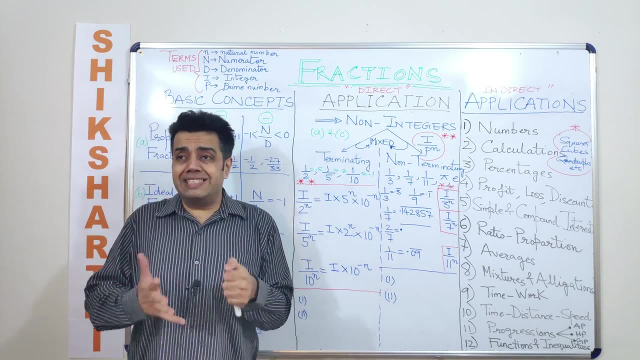 only So. once I start calculating these, then I feel the importance of calculations. And what do I mean by calculations? here is this: I should know the basic calculative things like how much is a square of a number, How much is the cube of the number? 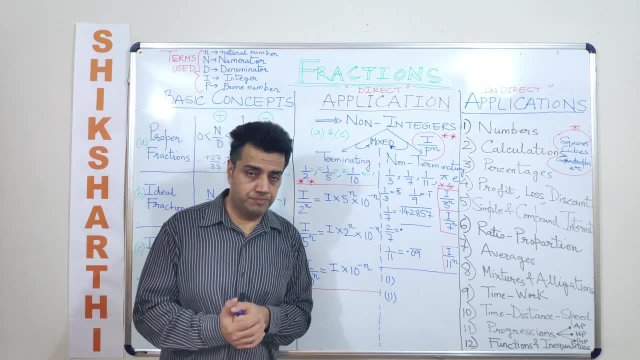 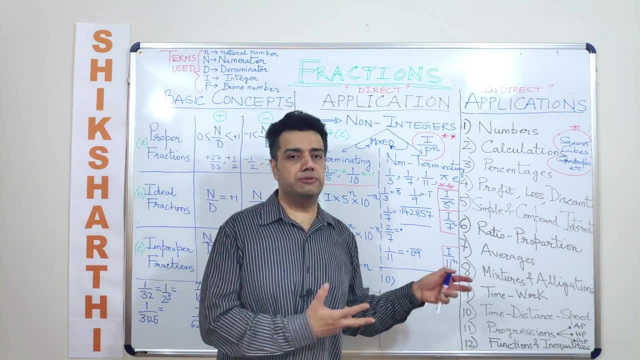 How much is the quadruple power, or a power five and henceforth? And I know the methods. We know the methods to calculate them. If you don't, you can refer to my videos which talk about these methods. Okay, So now. 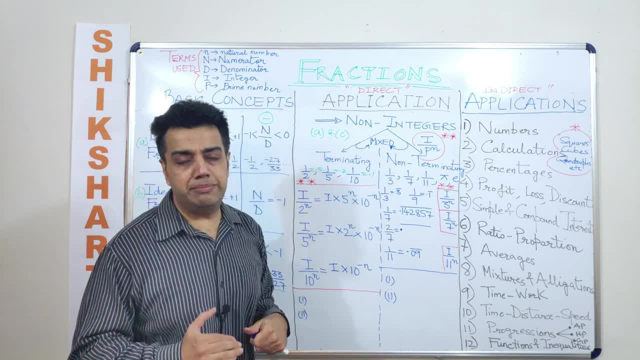 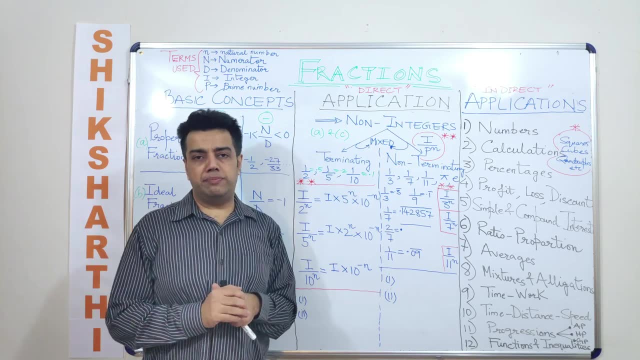 If I say one divided by two to the power five is one divided by 32, and I don't want to mug up how much is one by 32.. What will I do? I just need to calculate five to the power five. How will I do it? 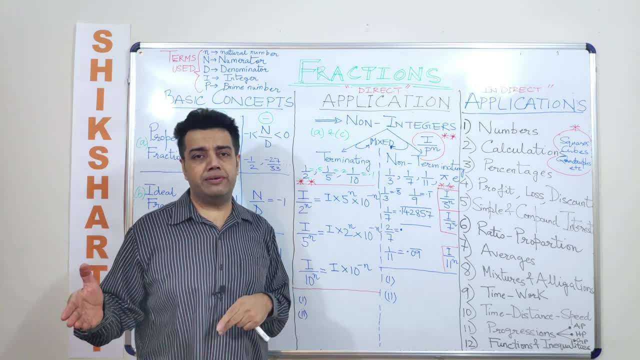 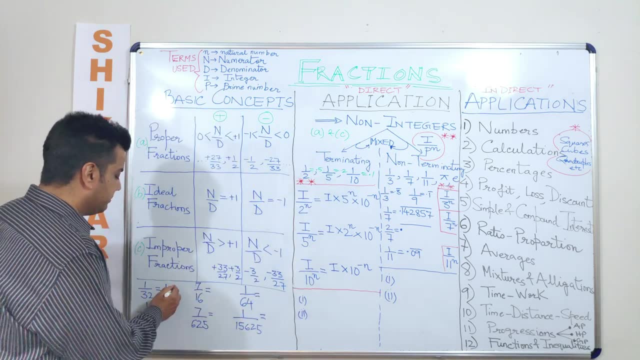 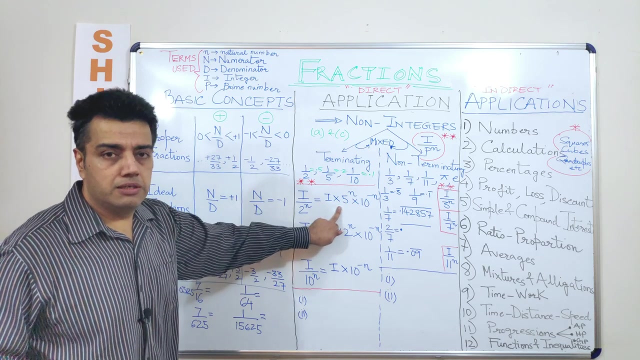 Five into five, 25 into five, 125 into five, 625 into five. three one, two, five. That means this can be written as point zero: three, one, two, five. with the help of this number, Where in the value of n is what. 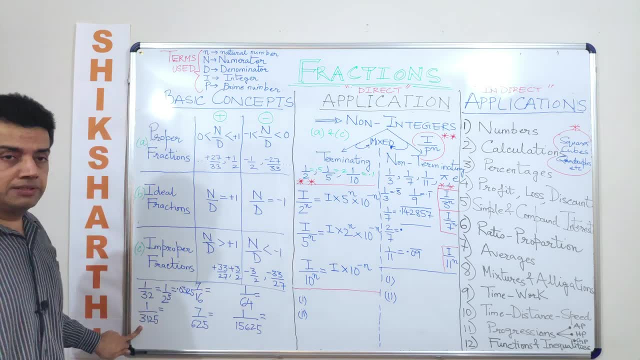 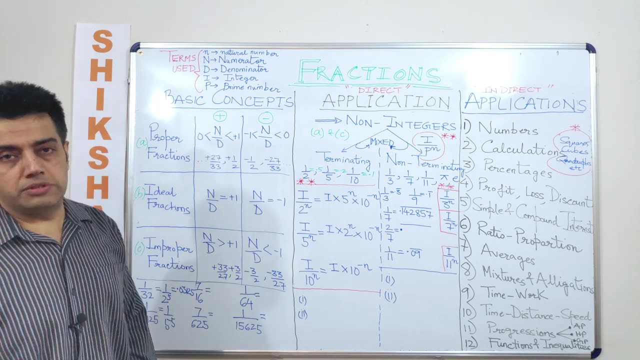 Five. Similarly, if I need to calculate this, half of the work I have already done few seconds back. only I calculated five to the power. five is how much three, one, two, five, Now one divided by five to the power five is just like saying one into two to the power. 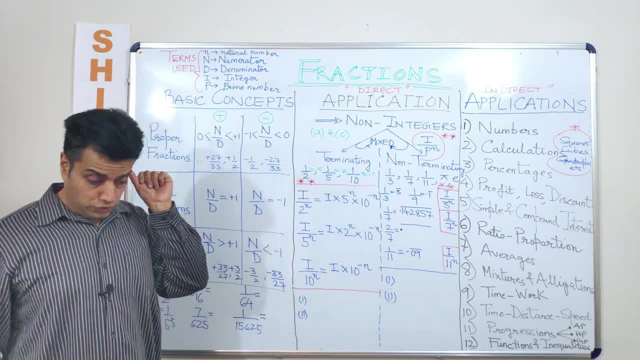 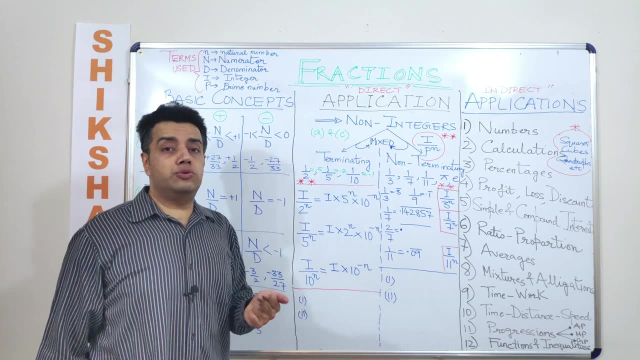 five into 10 to the power minus five. So what is the concept of 10 to the power minus one? You write the number, You shift the decimal point to the left hand side by one. What is the concept of 10 to the power minus two? 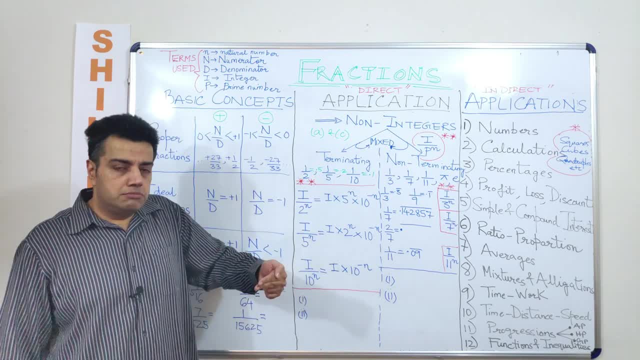 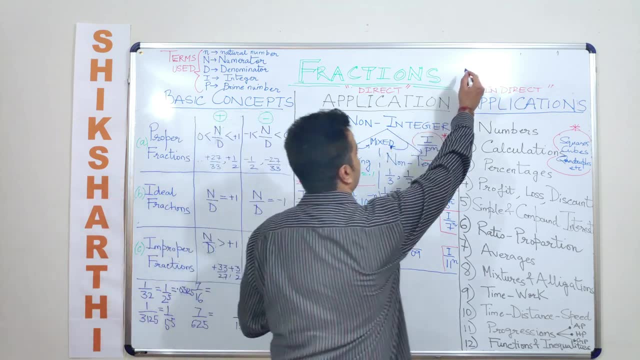 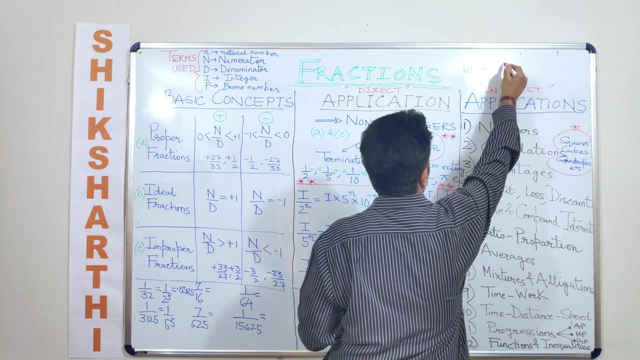 You write a number and shift the decimal. two sides, I mean two places to the left side. For example, if I have to write 10 to the power minus two is how much I'll write one and from here I shift the decimal here. 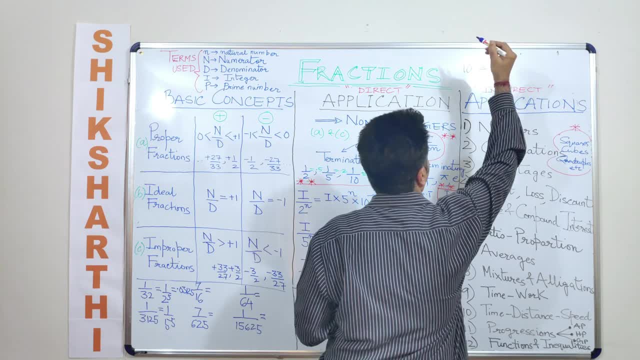 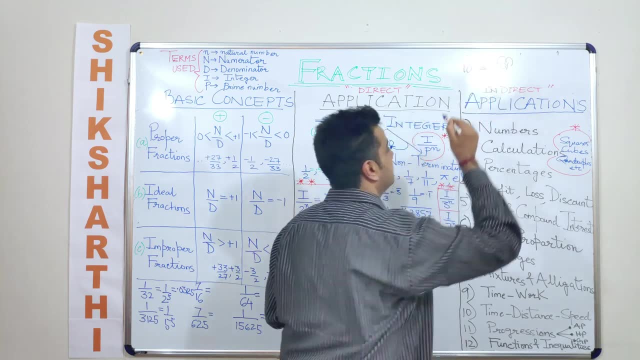 So I put a zero here and then I shift a decimal once again. Okay, So how many times have I shifted the decimal One from this side to this side? and the second time I shifted from this side to the other side. This is the concept of 10 to the power minus n, or 10 to the power minus two. 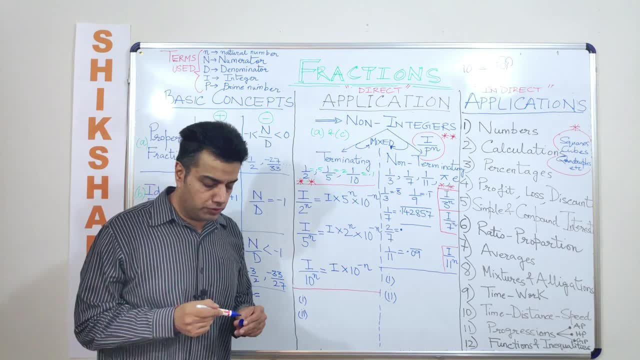 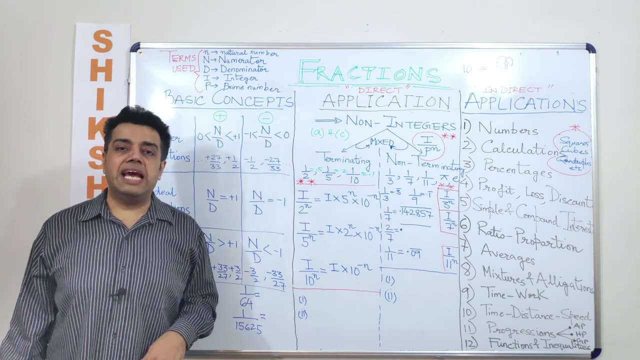 So, coming back, if I had to find out the value of one divided by three, one, two, five, what will I do? The moment, the very first thing I'm supposed to do is check whether this number is a power of five or not. 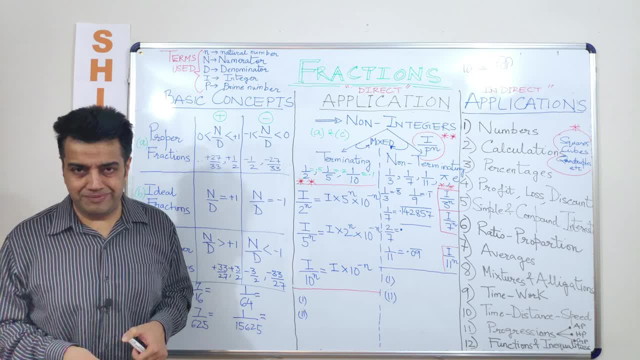 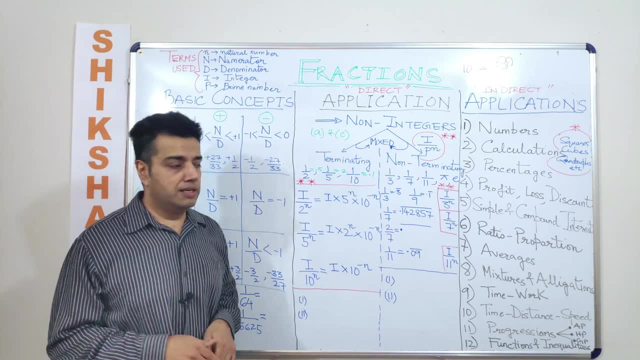 And the best way to identify this is because the number itself ends in a five. So any units, Any unit ending in the five may be a power of five or a multiple of five. But here I need to check whether it is a power of five or not. 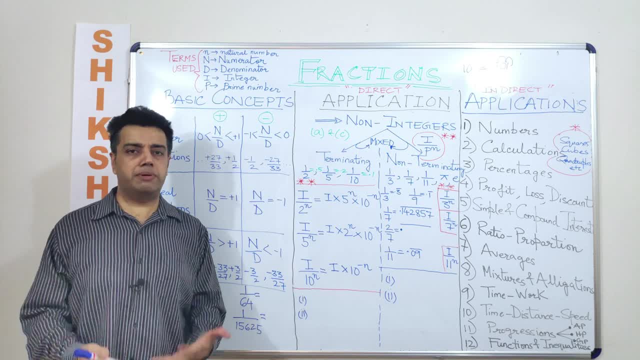 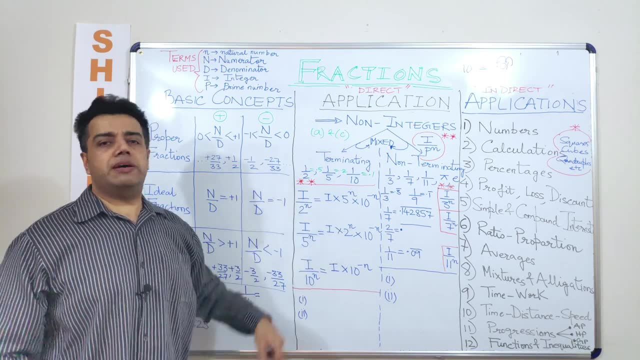 So we were able to find it out- because few seconds back only we did- that five to the power five is three, one, two, five, right? So in that case, one into two to the power five becomes how much two into two into two? 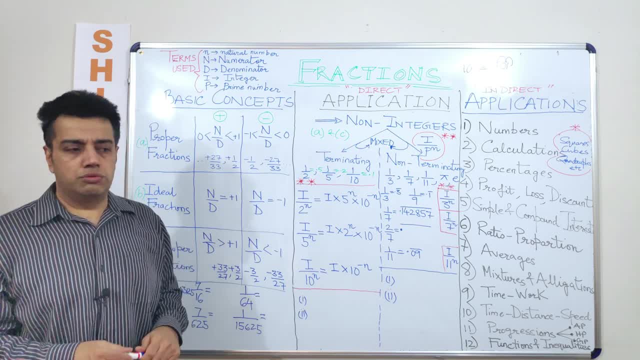 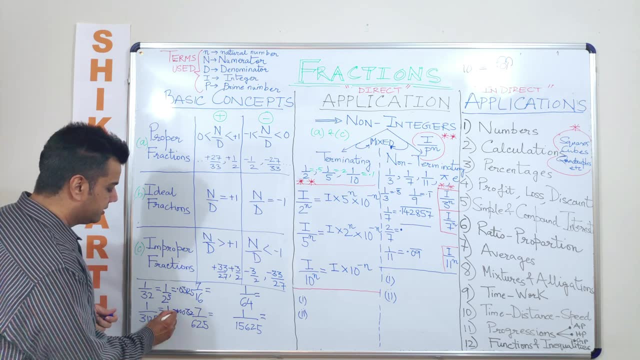 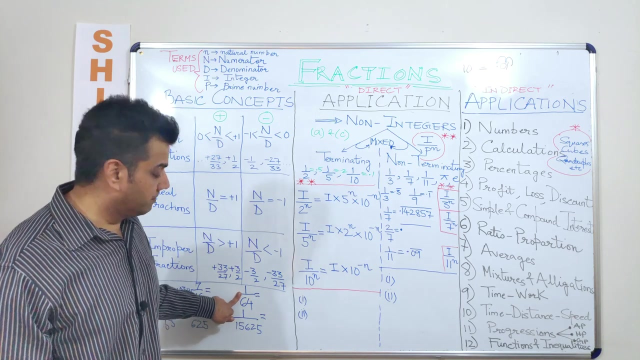 into two, 16 into two, 32.. Okay, Okay, Okay. So let's count. How do I make this as five digits? 0, 0, 0, 3, 2.. Similarly, I can do this. Similarly, I can do this. 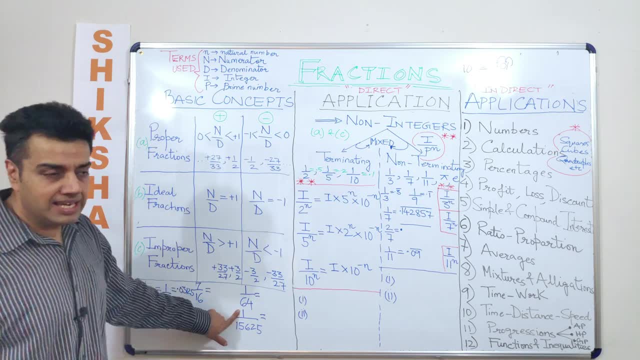 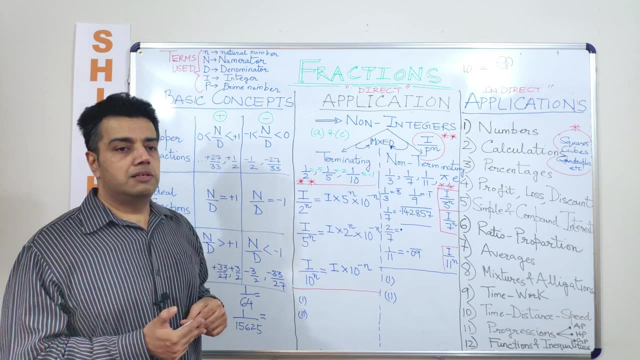 So let me choose one from here. For example, if somebody gives me a question like, calculate the non integer equivalent of one divided by one, five, six to five seems to be a difficult question, but it may not be. This may seem to be an easy question, but it may be difficult. 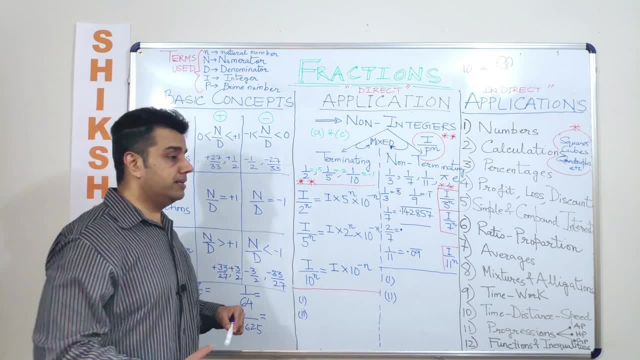 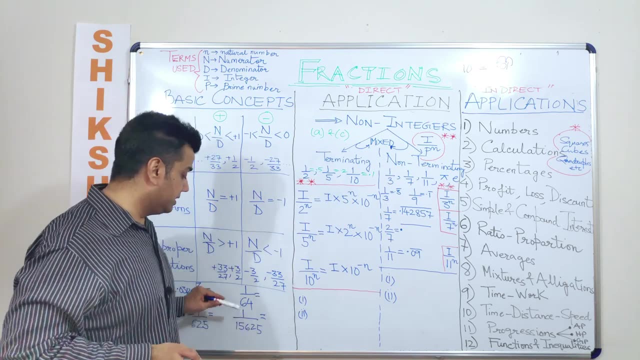 Right. So maybe I'm giving you a hint here. If the denominator is small, maybe the death, you know, the non integer equivalent may be difficult to find out, but if the desk, if, if the denominator is a bigger one, maybe. 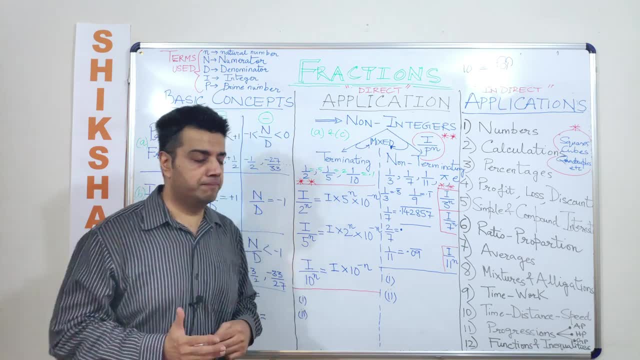 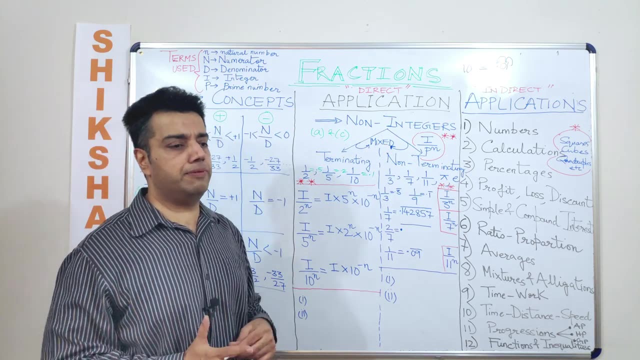 the non integer equivalent becomes easier maybe. So here again we have done half of the work. few seconds back, a few minutes back, we had found out how much is five to the power. five, five to the bar. Five is three, One, two, five. 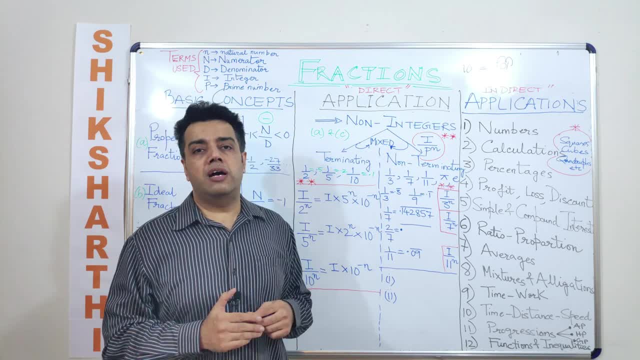 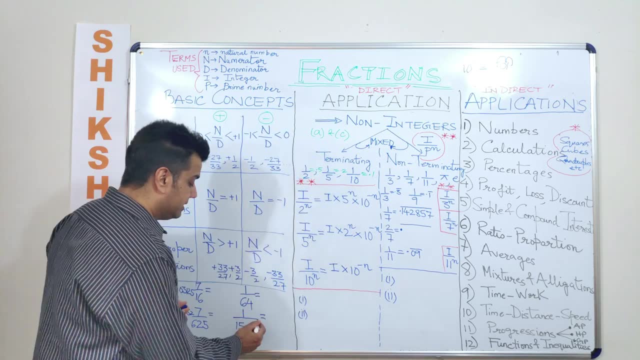 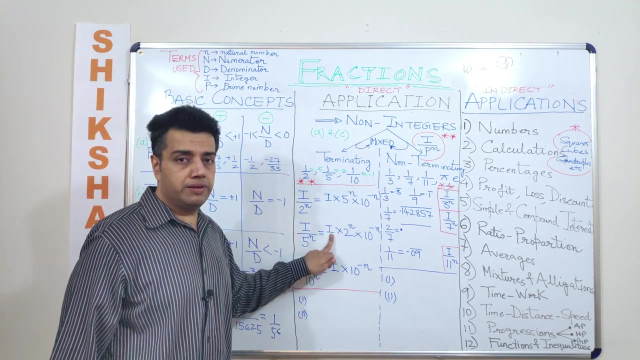 If I multiply it further by a five, how much do I get? one, five, six, two, five. In short, this is just like saying: this is one divided by five to the power six. Now, one divided by five to the power six essentially means what if I have to convert it into a? 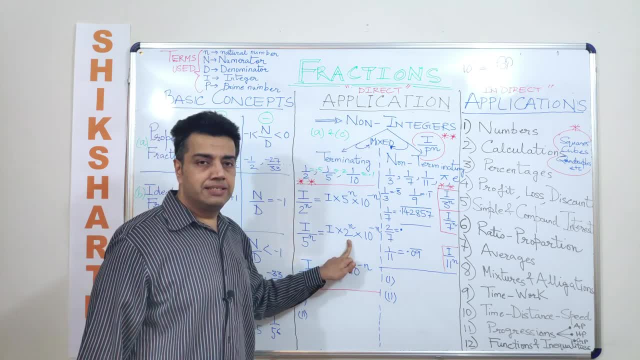 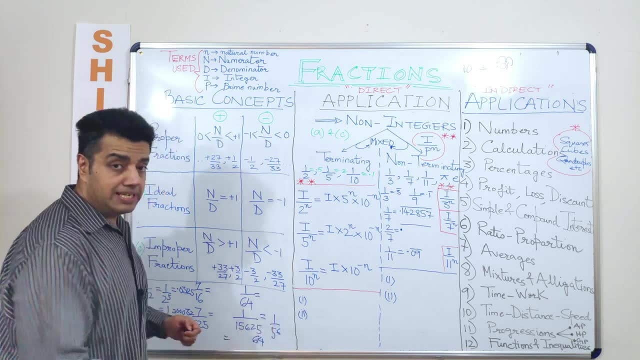 non integer. it means one into two to the power, six into 10 to the power minus six, which is just like saying two to the power. six is 64. Okay, And what is the power here? Six. So make these digits as six digits. 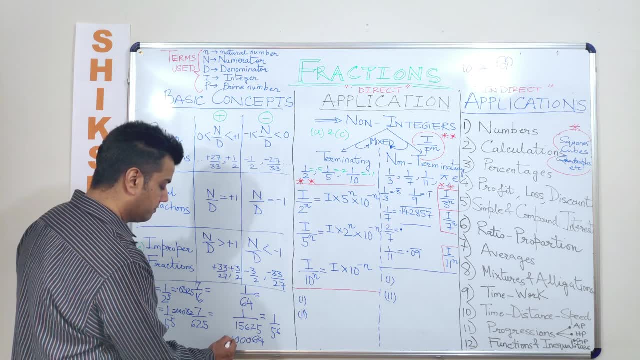 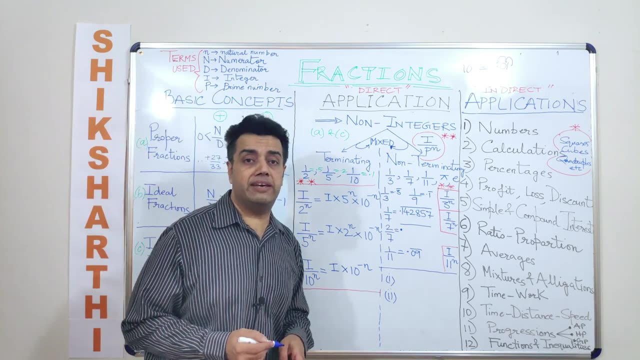 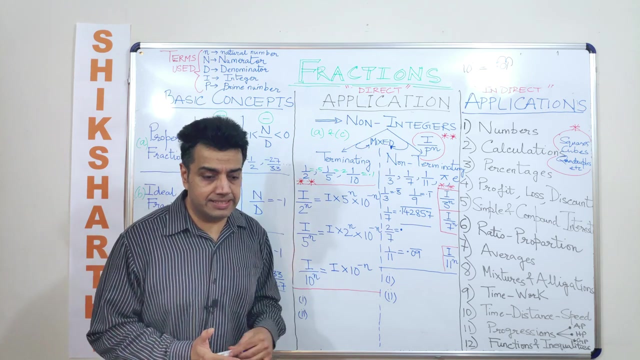 How do I make it And then put a decimal point here. See, so easy The remaining. you can do it for yourself. I hope I have motivated you enough, or I have mentored you enough, that now, after some practice, you should be able to take such kind of questions on your own. 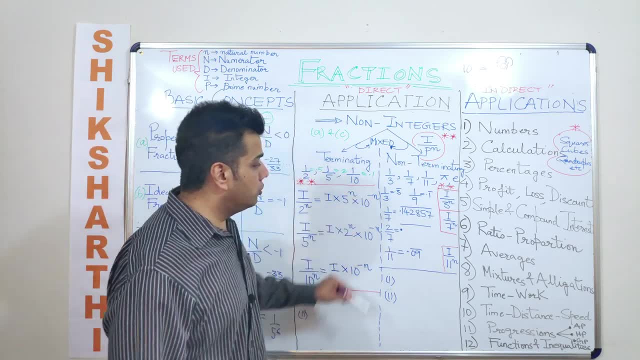 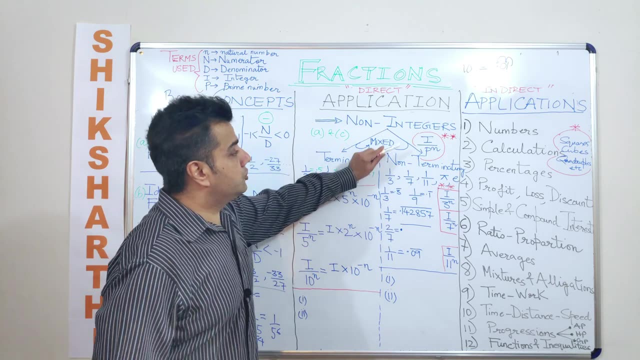 Now coming down to the recurring decimal part of it. Okay, So we all know, but now let us talk about the interesting part of all these things. So if I say any fraction which is written in the form of an integer divided by a prime, 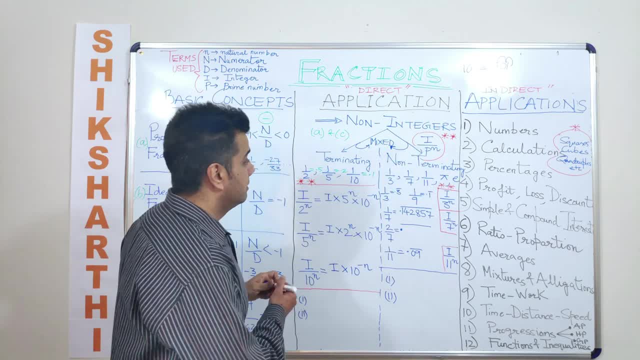 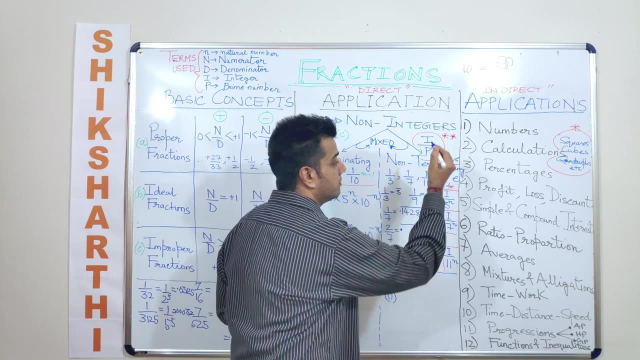 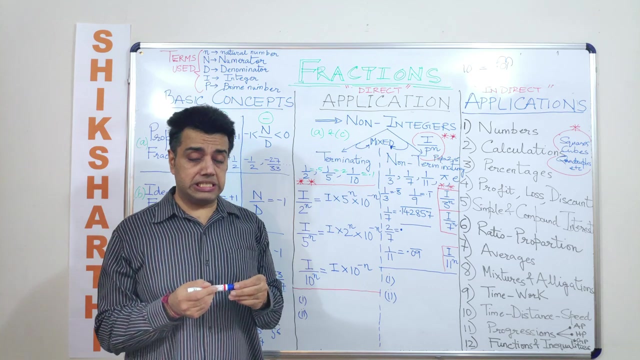 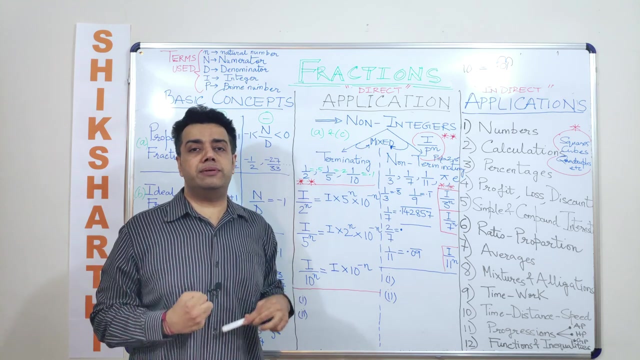 number, but this prime number to the power n. but this prime number should not be a two or five, because the moment it becomes a two or five, it becomes what? a terminating decimal or a terminating non integer Right. So when does a fraction yield a recurring decimal or a recurring non integer? A fraction will yield a recurring non integer only, and only if the integer- I mean the numerator- is an integer and the denominator is a prime number or a power of a prime number, but that prime number should not be either a two or a five. 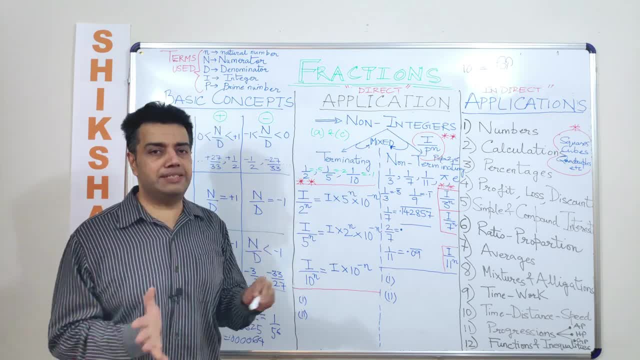 In that case, the resulting non integer or the decimal should not be a two or a five. Okay, So when does a fraction yield a recurring decimal or a recurring non integer? Right, A recurring decimal will always be a recurring non integer or a recurring decimal. 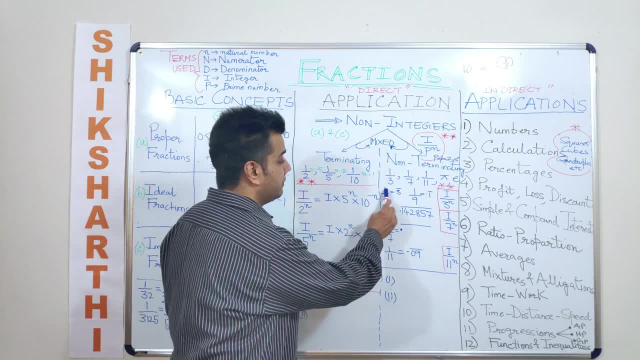 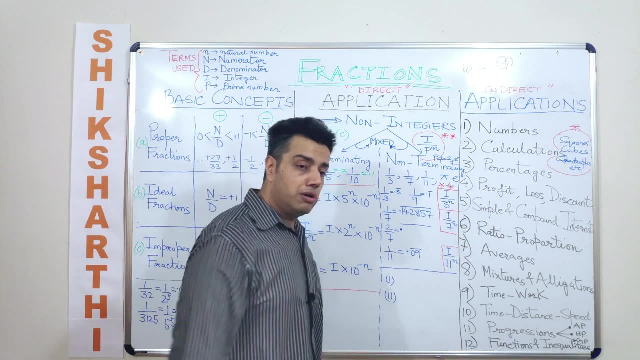 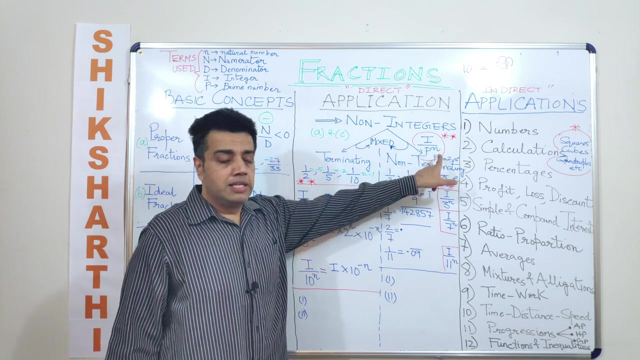 I hope this part is clear. Taking it forward Now, if I say one by three is going to give me a recurring decimal. So in that case, one divided by any power of three will always give me a recurring decimal only. Yeah, this is what we discussed few minutes back. 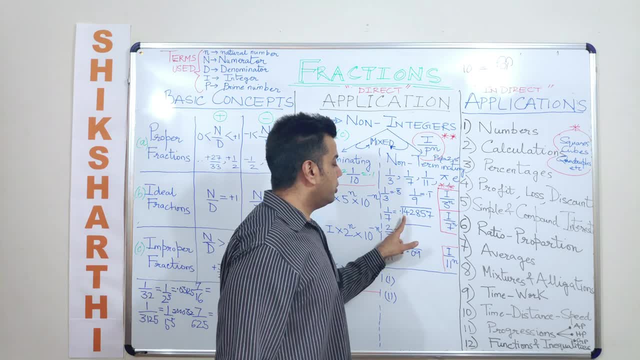 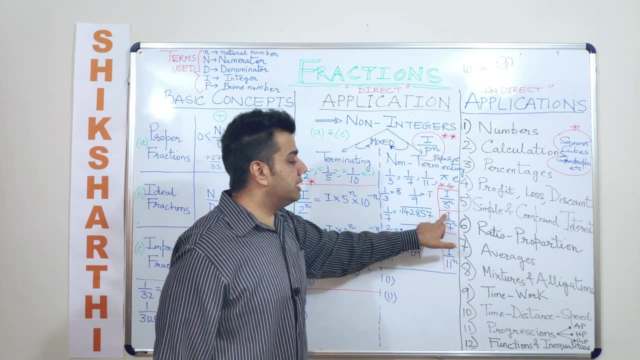 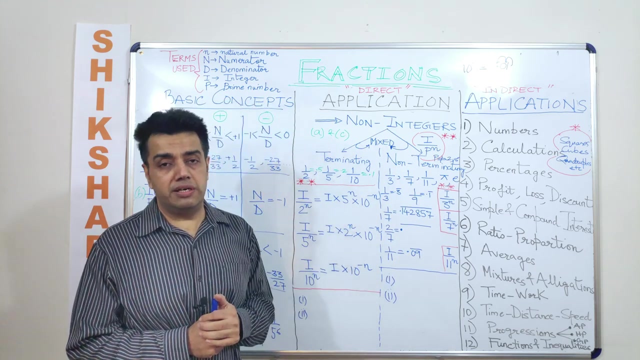 So if one by seven gives me a recurring decimal as 0.142857.. Right, Any number of the form or any fraction of the form wherein the numerator is an integer and the denominator is a power of seven will always give me what a recurring non integer. 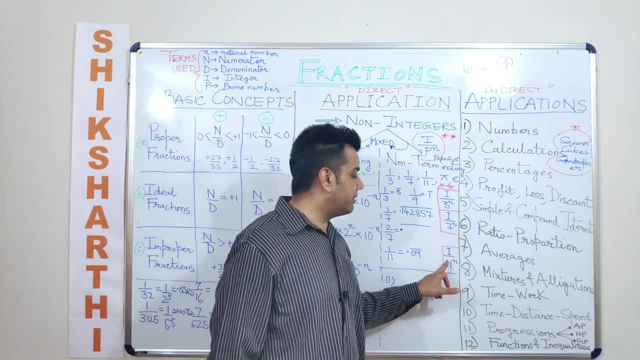 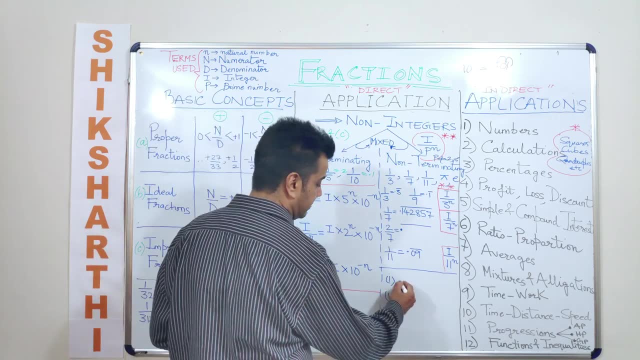 or a recurring decimal Same with: I, divided by 11, to the power n. So this is the first part that we have discussed. So we have discussed this first part. Now, what is the first part? I divided by p to the power n. 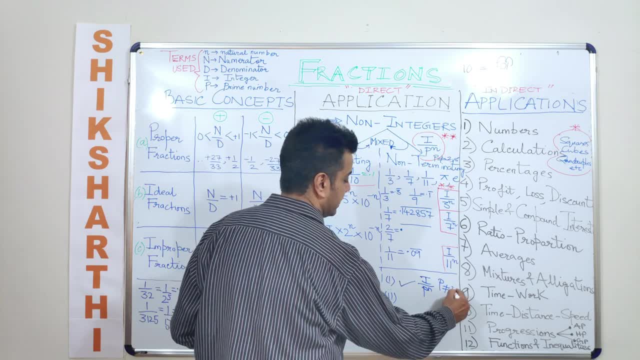 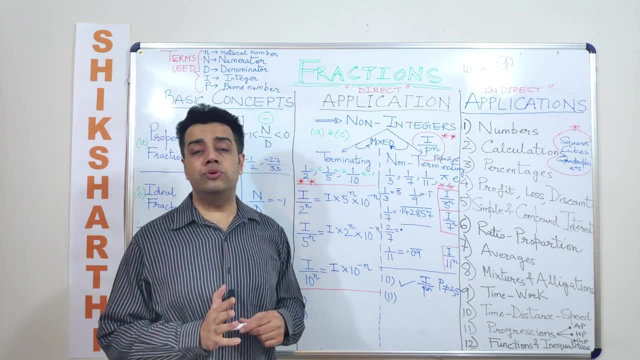 P to the power n, such that this p should not be either a two or five. where I is an integer, p is a prime number, n is a natural number. All such kind of fractions will always give you recurring decimals or recurring non integers. 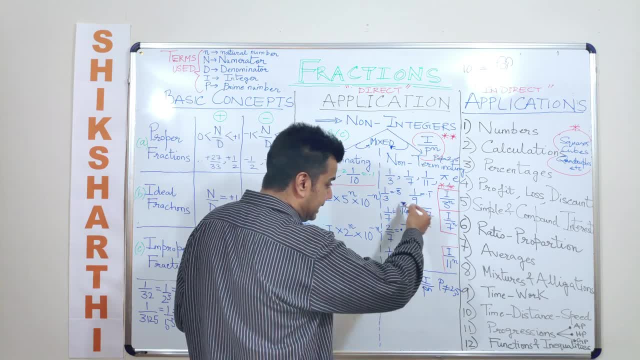 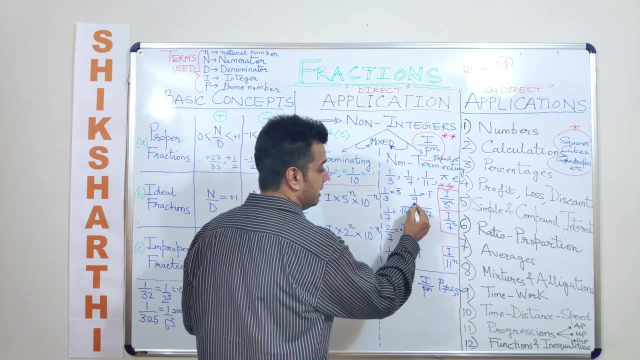 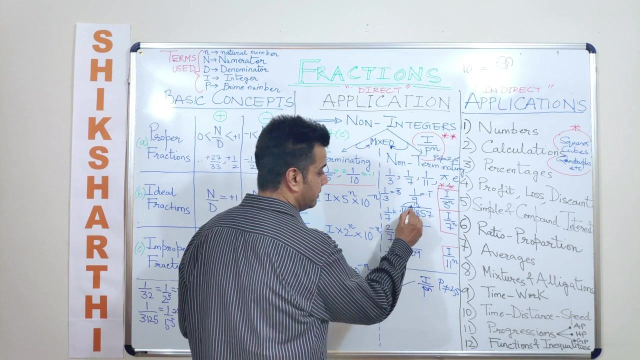 Second interesting part is if in the, if I talk about the recurring decimal here and if I'm getting even number of recurring decimals, even number of recurring decimals, let me bisect them, So you'll see something very interesting. And the interesting part is: one plus eight is a nine. four plus five is a nine two plus. 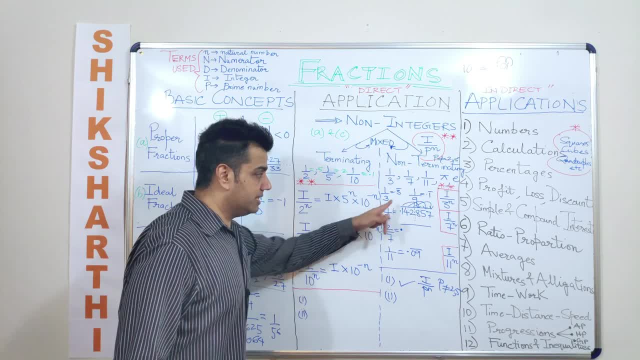 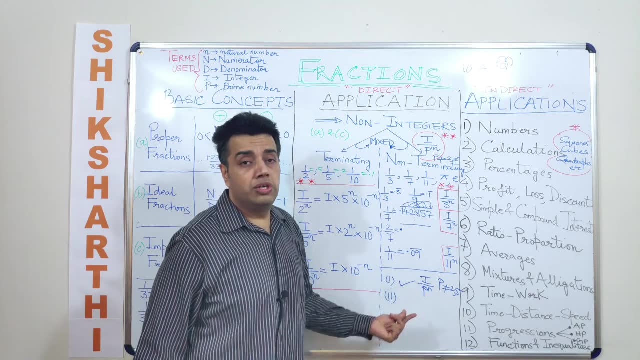 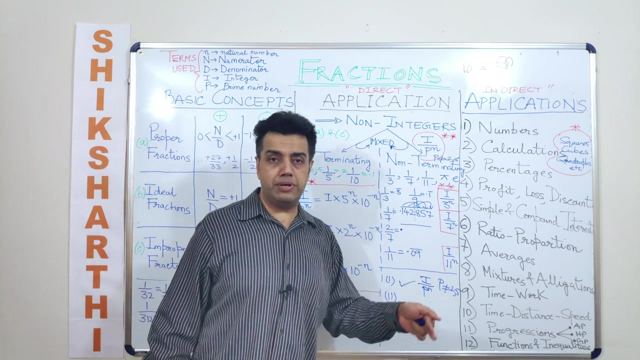 seven is a nine. I'll take this with the help of another example. Now, one by 11 gives me 0.09.. How many recurring decimal digits is it giving you? It is giving you even number of recurring decimal digits. So whenever I am getting even number of recurring decimal digits, let me bisect them. 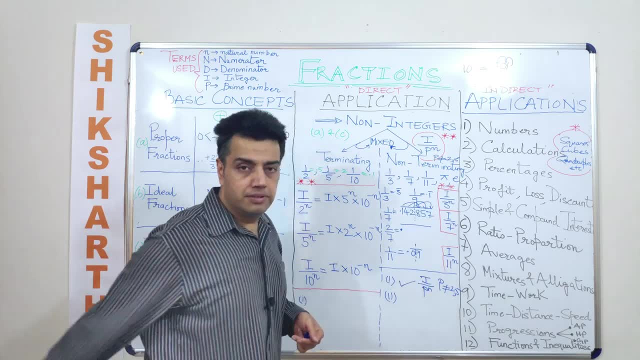 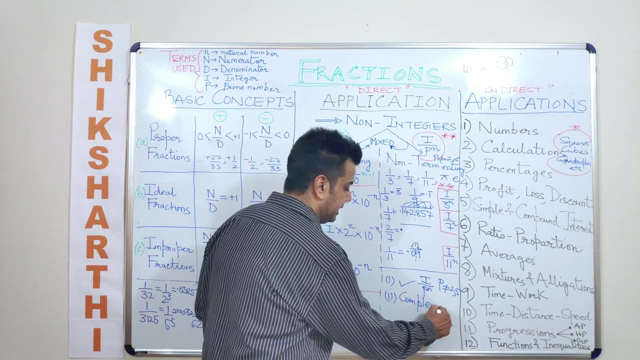 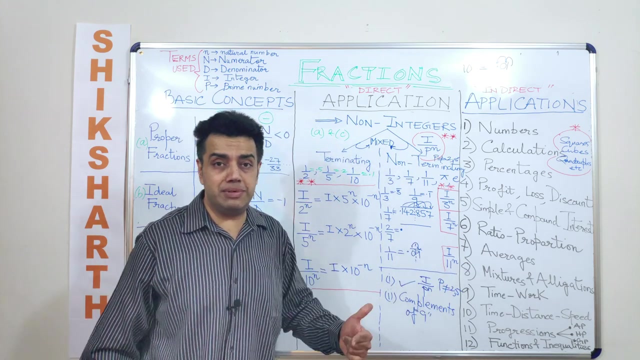 Bisect is dividing them into two equal parts, So then there'll be compliments of nine. This is the second interesting part that I discussed. The recurring decimals will be compliments of nine. after we would have bisected them, The recurring decimal digits will be compliments of nine. 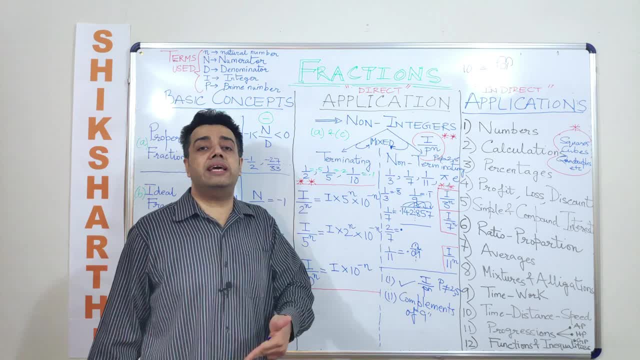 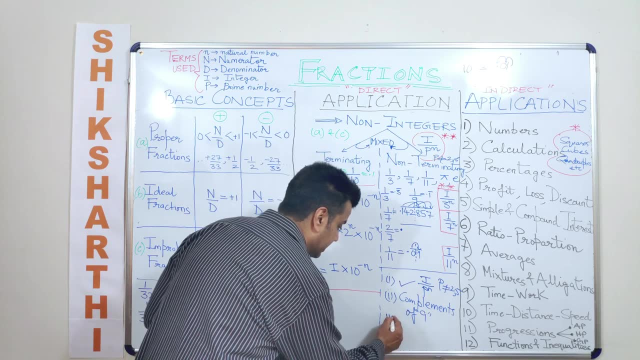 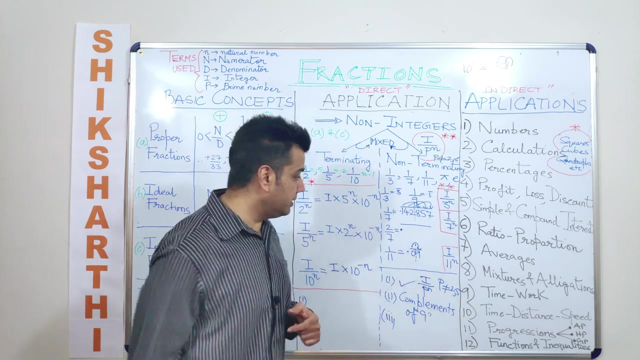 If we bisect them, and we can bisect them only when they have even number of recurring decimal digits. This is the second interesting part. The third interesting part here is: three into three gives me a nine. nine into one, gives me a nine. 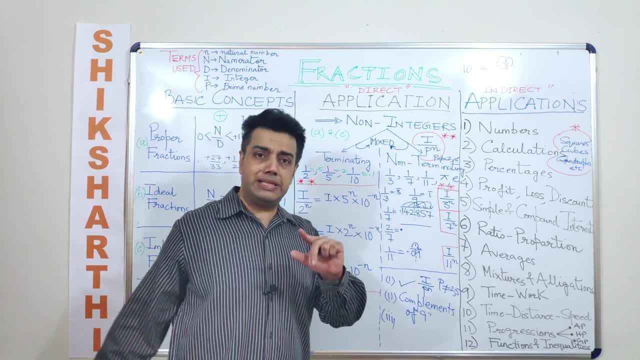 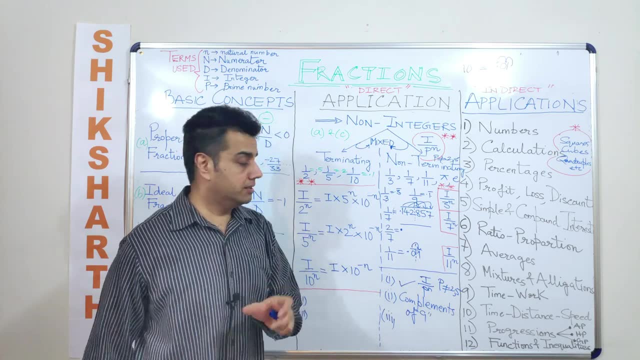 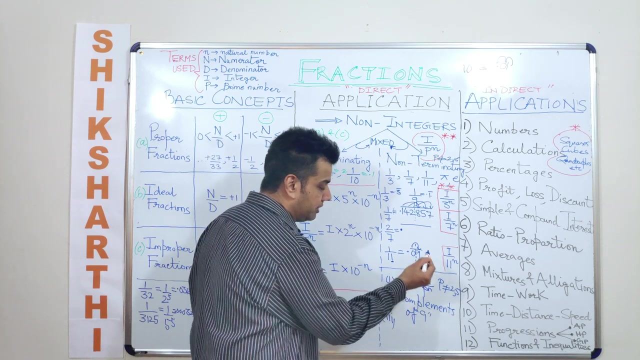 Now can I say this: seven into seven gives me a nine. Giving you a nine means what? Whatever number you are getting, that units digit of that number will be a nine. Similarly, the units digit of the fraction, the denominator of the fraction when multiplied. 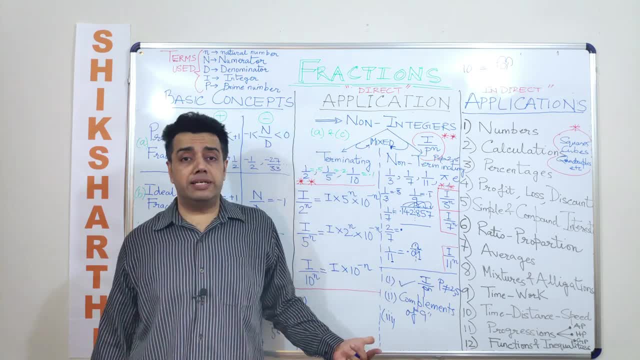 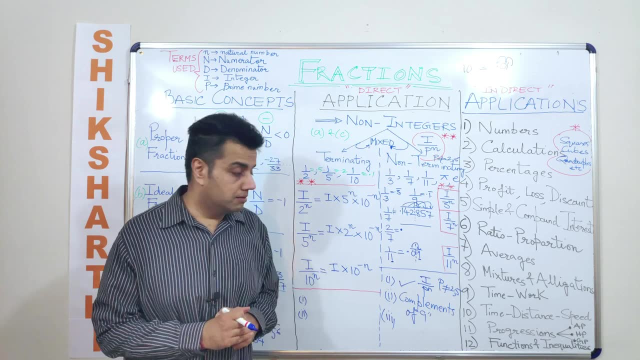 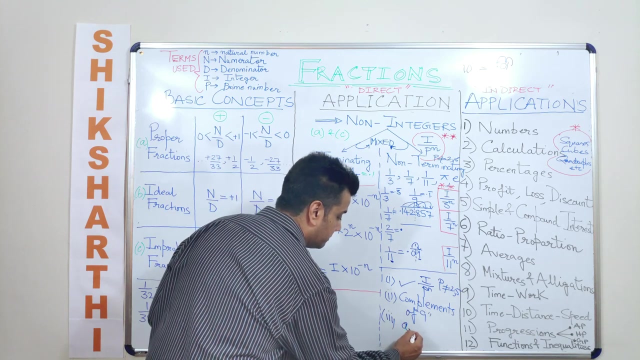 with the units digit of its decimal equivalent, which is a recurring decimal equivalent, will always give me what It will give me: a nine. So if I say the units digit here, the units digit here, let's say this is a naught and 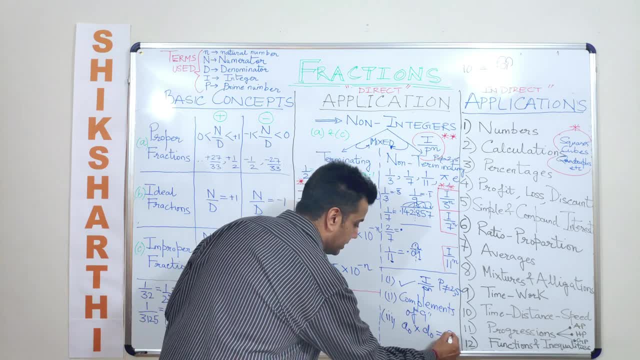 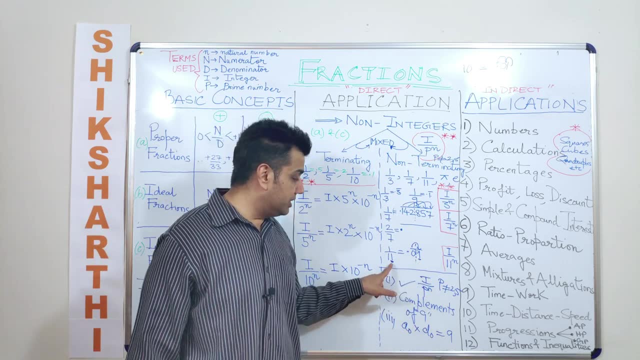 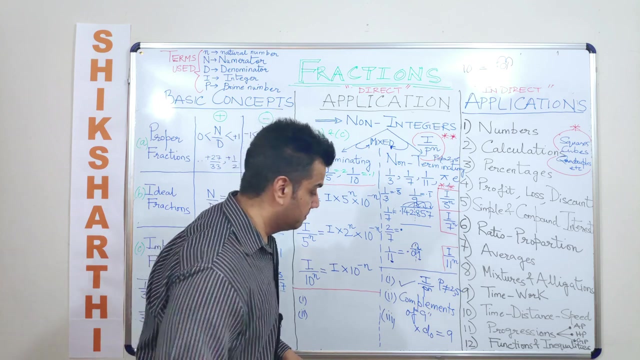 the units digit here, which is D naught, will give me a nine that this D naught is the decimal equivalent units digit. Okay, So in this we are talking about the denominators units digit. So instead of a naught, let me write it as capital: D naught. 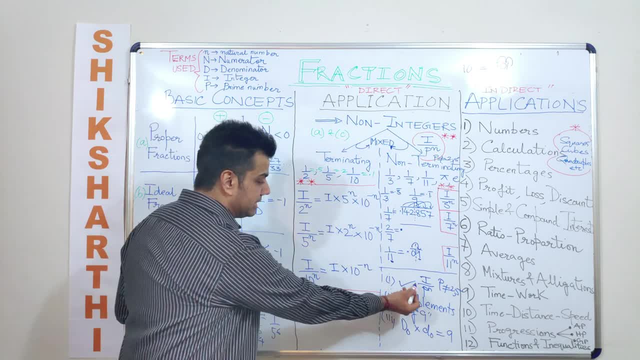 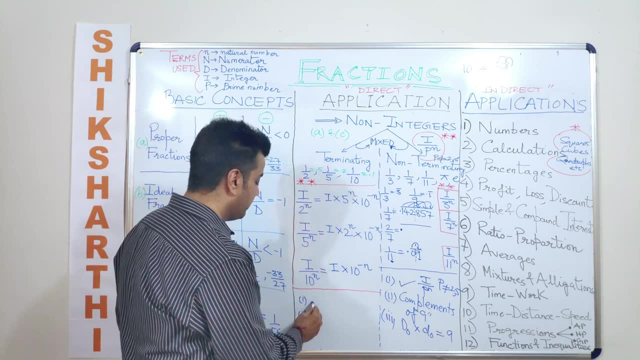 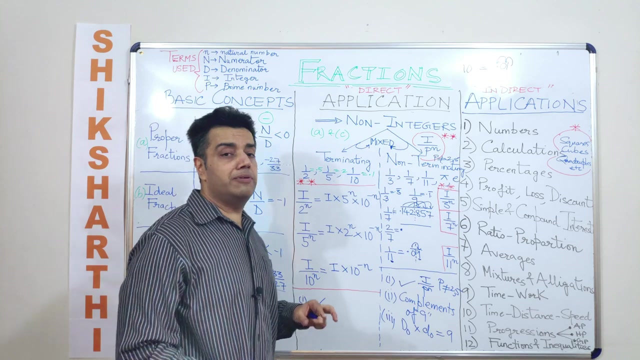 You will always get this. analogously, You can talk about the interesting parts here as well. So a terminating fraction becomes, converts into a terminating decimal when, when the denominator is when the numerator is an integer and the denominator is either a power of two. 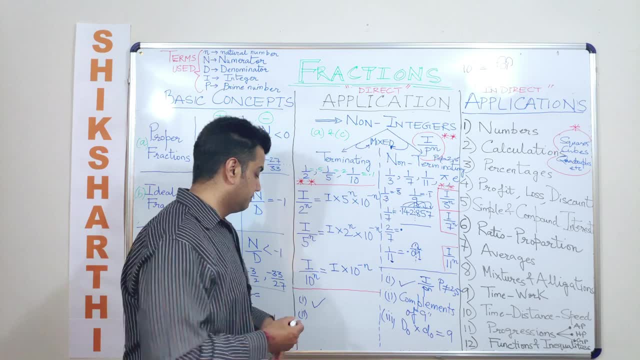 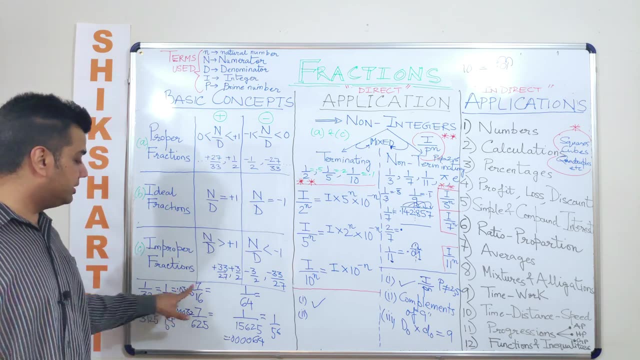 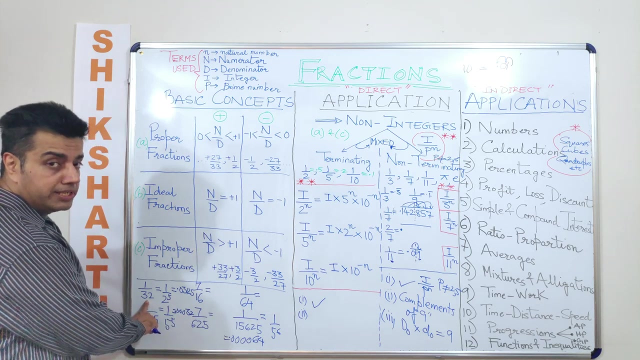 or a power of five or both of them. these are the three cases that we have already discussed. And then, taking the help of these examples that you had taken- because all these examples are the examples of terminating decimals- If I see the units digit of the denominator and I multiply the units digit of this denominator, 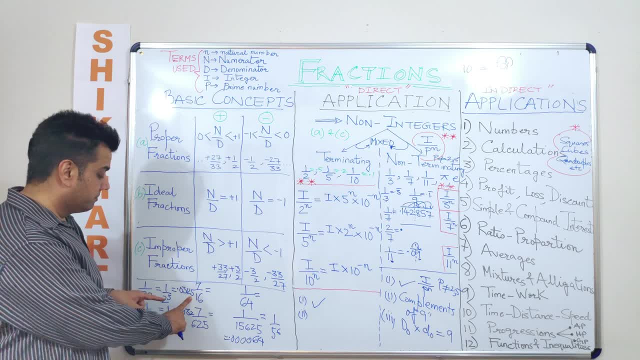 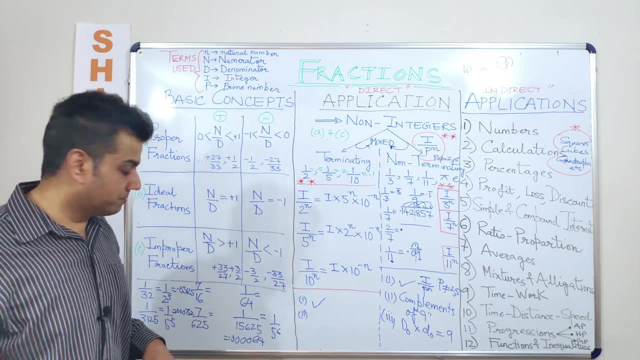 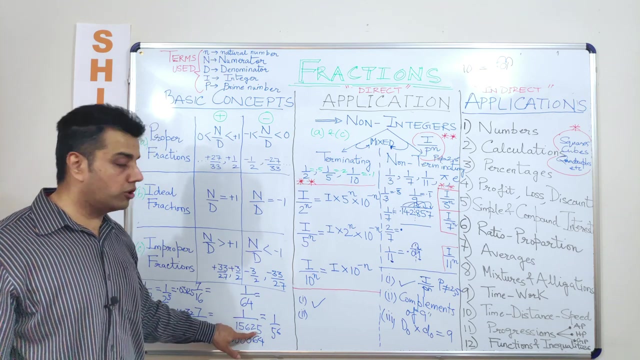 by the units digit of its decimal equivalent, which, incidentally, here is a five. So five into two gives me a 10.. 10 means zero in the units place, Same here. So here I, in the denominator, the units digit of the denominator, had what five and the units. 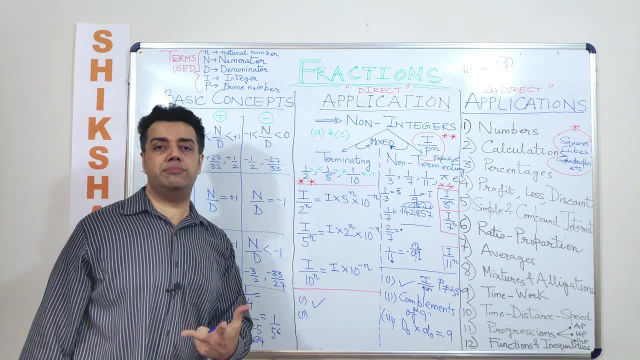 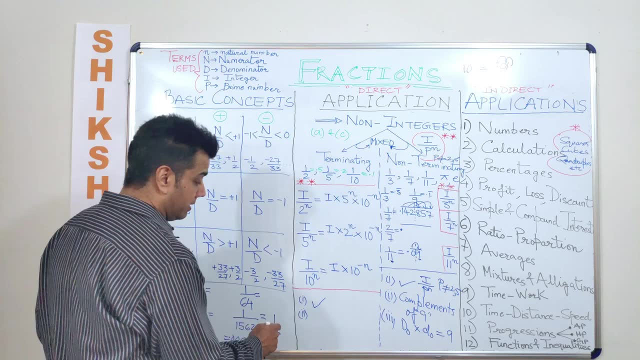 digit of its decimal terminating decimal equivalent. gave me what four, how much is five into four, 20, which gives me a zero. So you get the interesting part here as well. So which, incidentally, is this is what we are talking about. So, in case of a terminating non non-integer or a terminating non-integer, 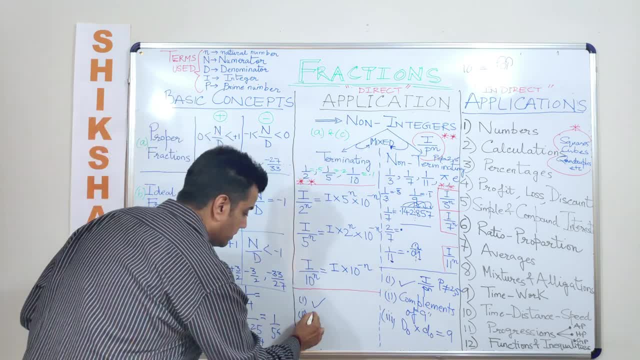 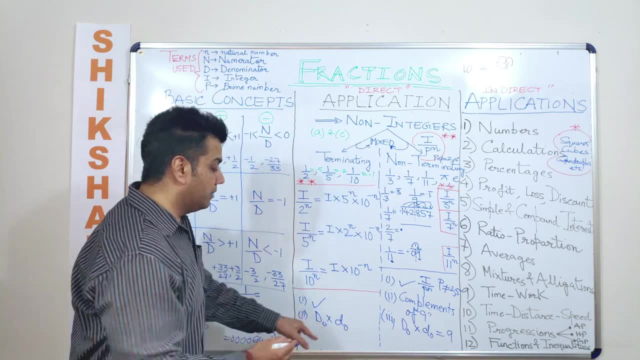 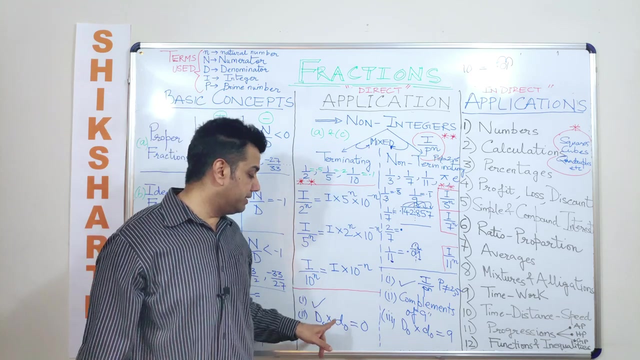 Okay, Before I talk about a terminating fraction, the units digit of the denominator, when multiplied with the units digit of its decimal equivalent, will always give me what a zero. This can be used as a test for terminating fractions, and this can be used as a test. 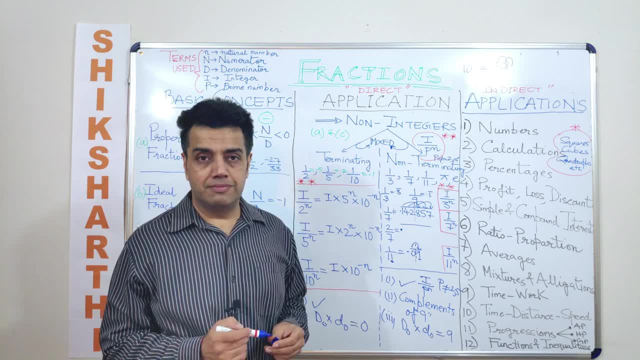 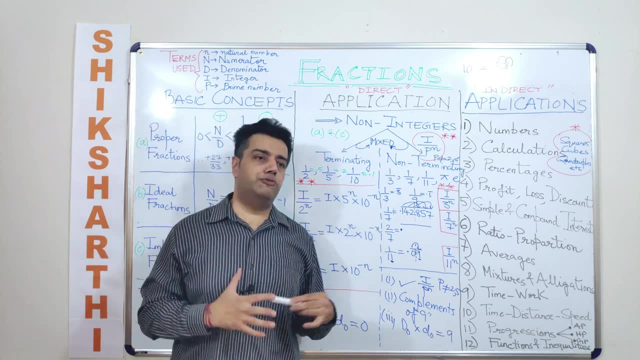 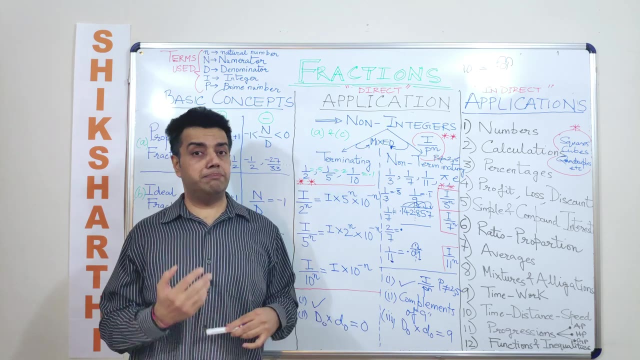 for recurring fractions. I hope. I mean this is too much of things to be processed. I hope, If you spend somewhere around one hour trying to revise what we discussed here, the things become simpler. So now taking your learnings to the final stage, which is indirect application of this. 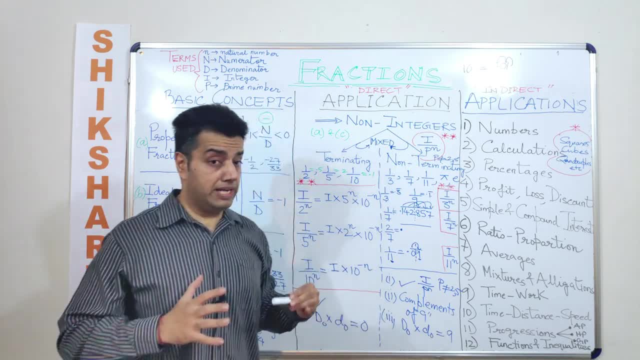 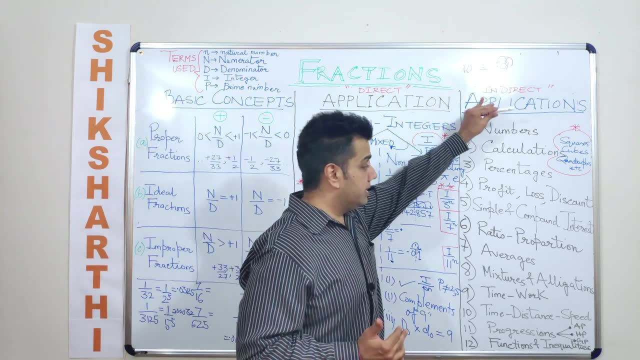 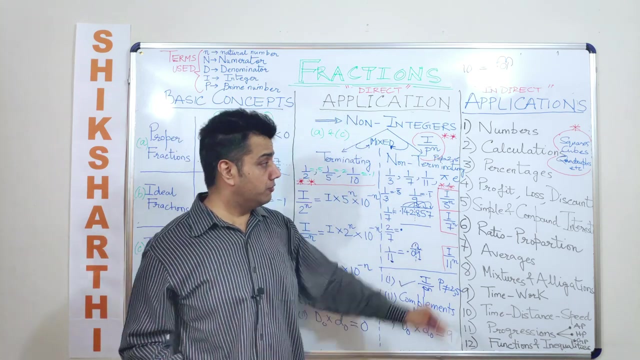 topic. So, if I talk about our fractions important- yes, they are very, very important because they have a direct application and then they can be associated with all of these topics. And how many topics? 12 of them. I have not written all of them.